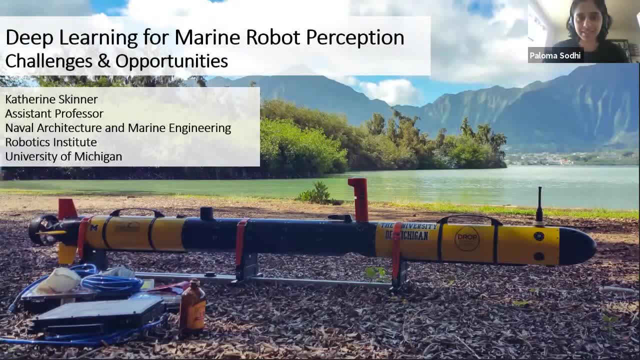 So hi everyone. Today we will be hearing from Catherine Skinner. Catherine is an assistant professor in the Department of Naval Architecture and Marine Engineering and the Robotics Institute at the University of Michigan. She's also the director of the University of Michigan Field Robotics Group. Her research spans robotics, computer vision and machine learning, focusing 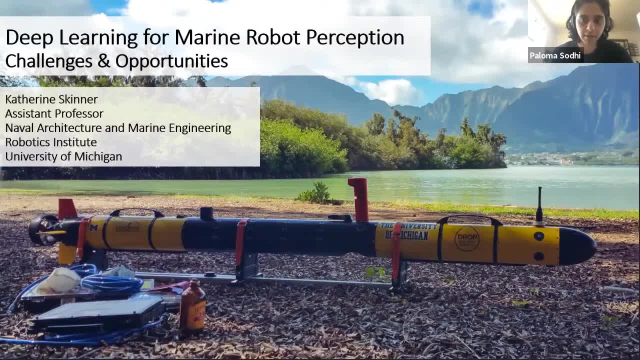 on enabling autonomy in dynamic and unstructured environments across field robotics applications such as underwater exploration and autonomous driving. Her field work has taken her to many exciting locations, ranging from Sydney to Hawaii to Jamaica. She completed her postdoc at Georgia Tech and her PhD from the University of Michigan Robotics Institute, where her research received. 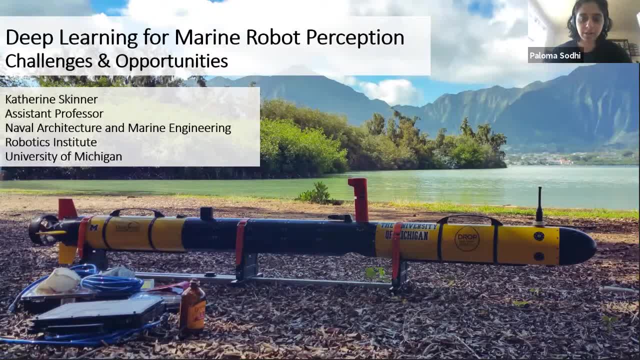 the outstanding honorable mention. Today she will be talking about her research on deep learning for marine robot perception. With that, I yield the floor to you, Catherine, Thanks. Thank you for the introduction. I'm excited to talk to you all today about deep learning. 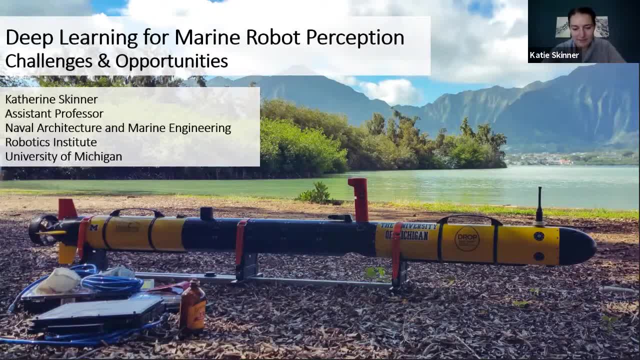 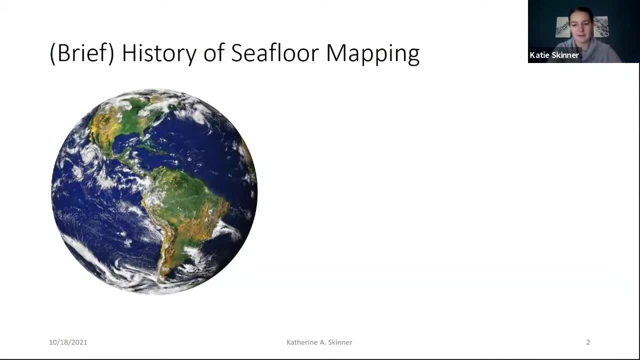 for marine robot perception And throughout this talk I want to take a chance to highlight some challenges for marine robotics and opportunities that we have to push the field forward. So I'd like to kind of start by taking a step back to give you kind of see where the robots 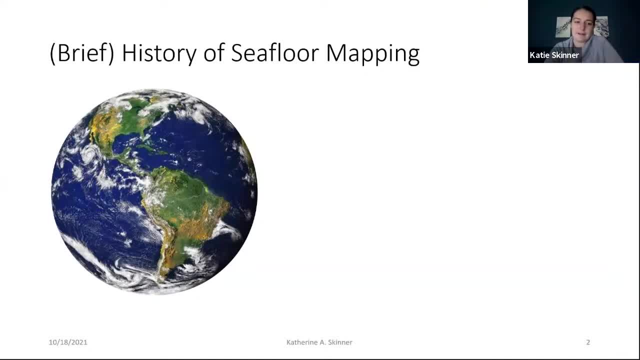 sit in the context of sea floor mapping by looking at a very brief history keyword: sea floor mapping. So marine environments make up 70% of our planet And for centuries humans have sought to explore, map and understand these environments And we've come up with 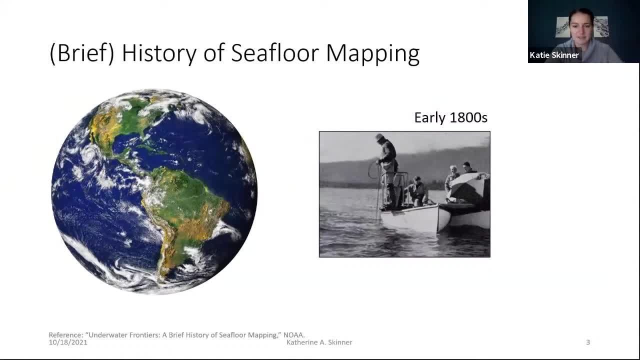 more and more advanced ways to do this over the centuries. So if we look back to the early 1800s, some of the first methods to map the sea floor, map the symmetry, are these lead lines. These are actually lead tied to the end of a rope And surveyors would move around the 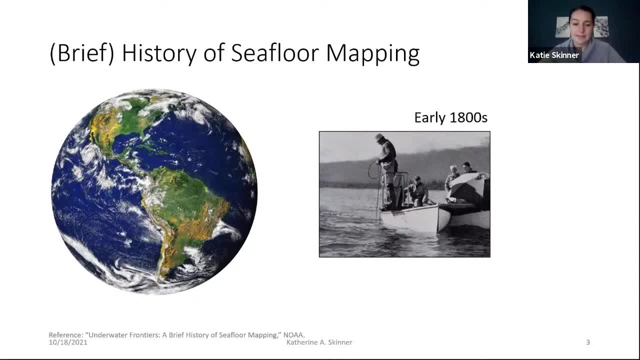 sea floor, drop the lead lines and measure how far they sink to the bottom. So you can imagine if we had to map 70% of the earth this way. this would take quite a long time. So luckily we've come up with more advanced technology throughout the years to allow us. 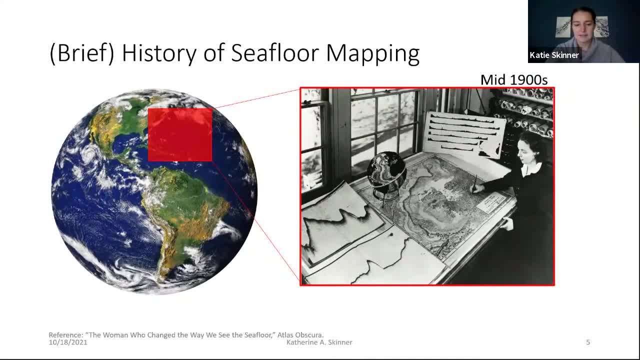 to collect higher resolution maps of the sea floor. This is in fast forward to the mid 1900s. Marie Tharp, who was a geologist and a cartographer and is commonly known as the women who mapped the sea floor. she was able to take sonar profiles of the sea floor and 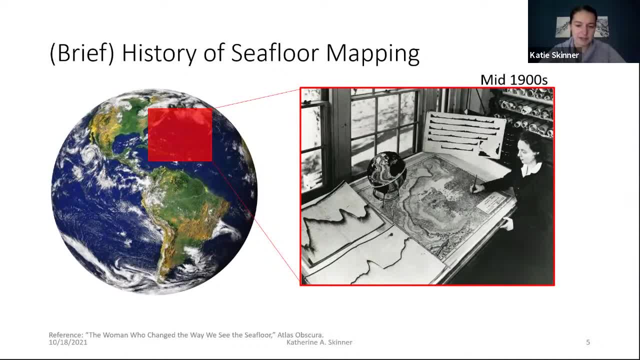 align them to ship tracks from the ships, collecting the sonar data, and draft very high detail maps, So drawn by hand, based on these sonar profiles. So we were able to get more and more information in higher resolution of our map, but still this is a very manual process. 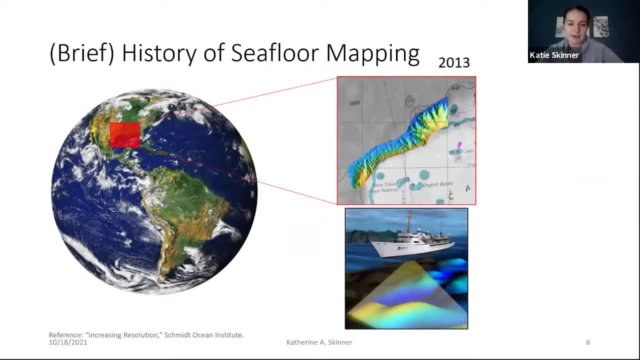 And if we think about current day technology- so this is from a survey in 2013,- so modern day, we now have sensors and tools that can allow us to complete these high resolution mapping effort with much more accuracy and with much less manual drawing involved, thankfully. 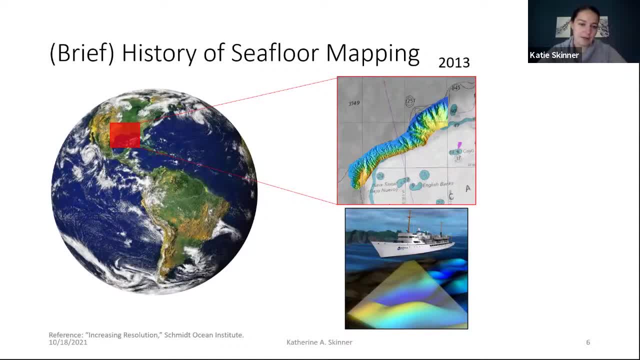 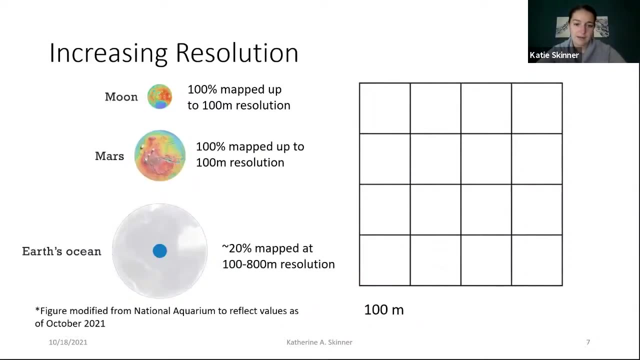 So you can see that this is a map from a multi-beam sonar that was mounted on a ship and this is a survey near the Gulf of Mexico, And with these surveys we can collect very high resolution structural information about the sea floor. But we still have really a long ways. 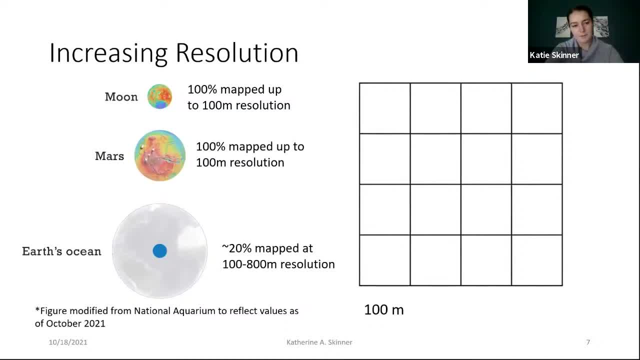 to go. so it's commonly referenced that we know more about the Moon and Mars than we do about our own sea floor, And what that really means is that we have higher resolution maps of the Moon and Mars than we do of the sea floor here on Earth. So both Mars and the Moon are 100%- almost 100%- mapped. 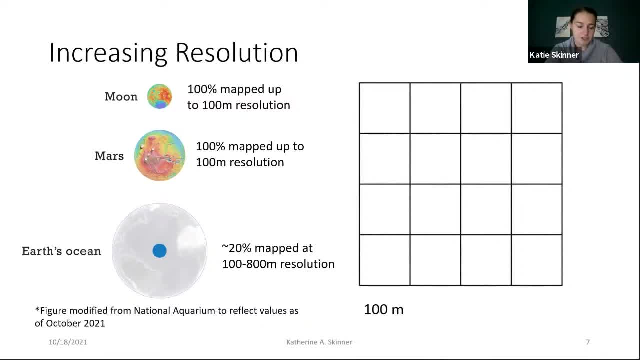 up to about a 100-meter resolution, but Earth's ocean is only about 20% mapped at a range of 100 to 800-meter resolution And you can think if we had a grid map at 100-meter resolution, there are still quite a few features that we might miss If we're trying to do detailed surveys. 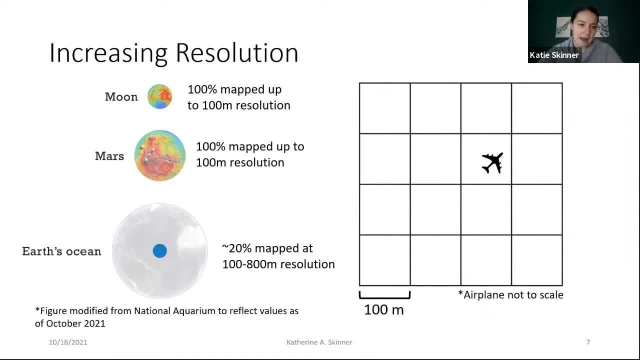 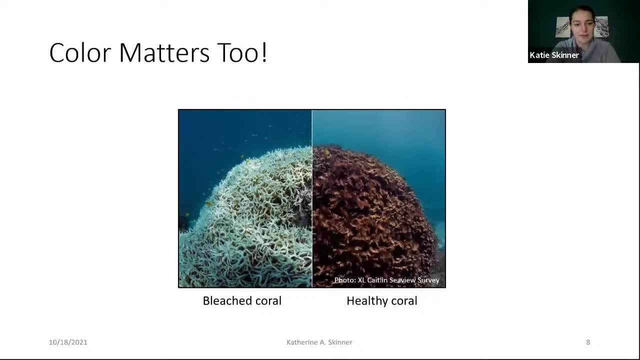 of the sea floor or if we're trying to identify objects that are smaller than this resolution, we still are going to face challenges in what we can see and understand in ocean exploration. On top of this, structural resolution isn't the only thing that matters. 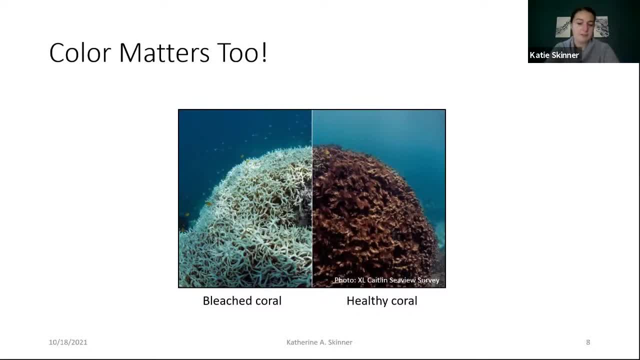 So for a lot of applications, color also matters too, So I've collaborated a bit with marine biologists, and they're interested in studying changes in coral reef systems over time, And for scientists, color of coral reef systems can be an important indicator for health of the reefs, So it's important to be able to observe and measure. 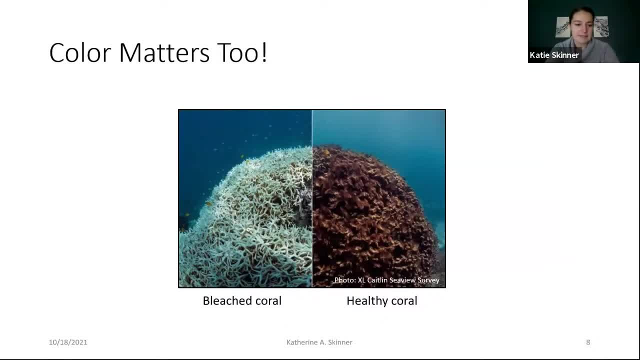 the color of these environments as well. As you can see on the right some healthy coral which has polyps that live on the coral. They have a symbiotic relationship. When the coral becomes stressed, it expels the polyps, leaving just the bone structure of the coral itself. 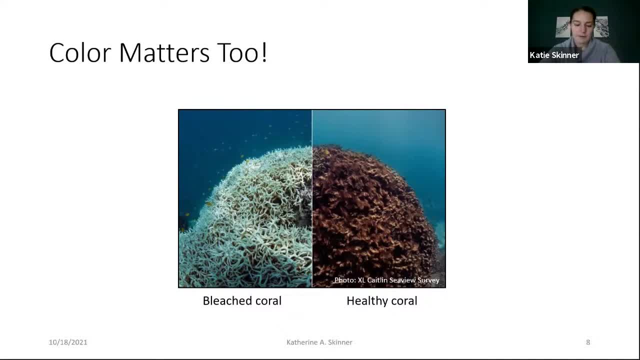 which is referred to bleached coral. So again, structure is one cue, but color is important too. And still, the main mode of sensing that we have for observing color, whether it's on land or underwater, is using cameras, And cameras, of course, are not new. But what is relatively new? 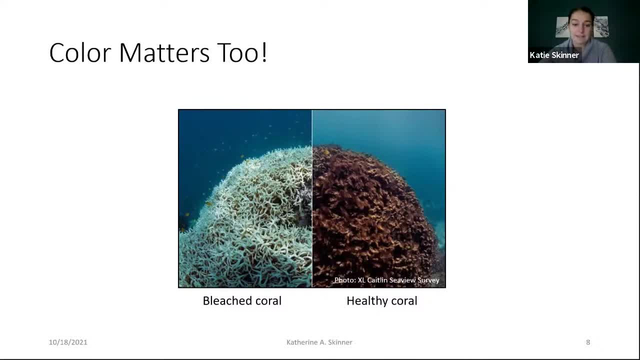 is our ability to bring cameras to the deep sea, So we're able to bring cameras to the deep sea and we're able to bring them to the surface of the ocean. And so we're able to bring them to the deep sea and we're able to bring them to the surface of the ocean, So we're able to bring them to the. 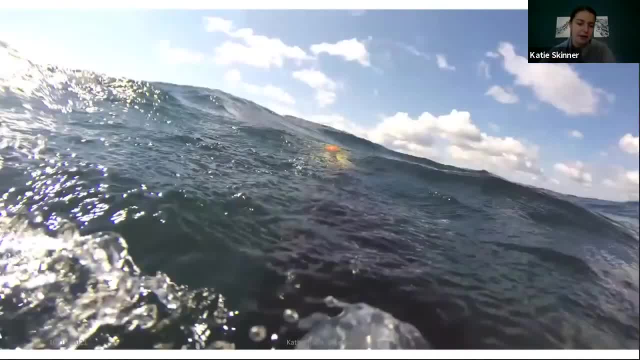 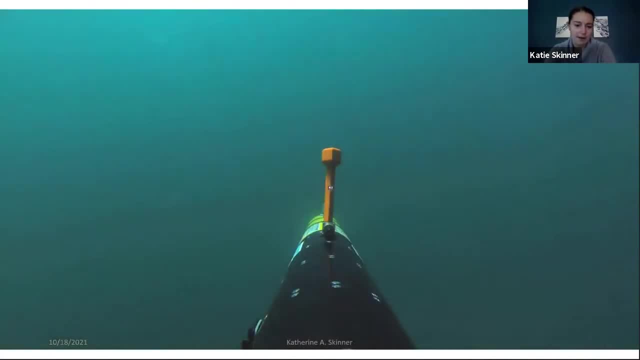 depths of underwater environments. So now we have the ability to attach cameras to underwater robots, like this autonomous underwater robot here surveying the Great Lakes, And we can send these cameras to the bottom of the seafloor. So robots equipped with imaging sensors can provide high 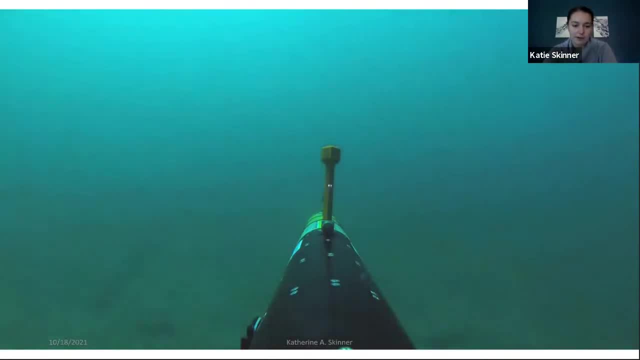 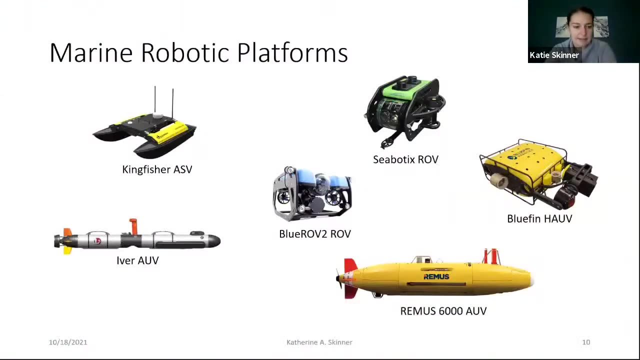 resolution: colored views of the seafloor all the way up to the full depth of our ocean. So it's been really exciting in recent decades is that more and more commercially available marine robot platforms are becoming available for lower cost: low cost, but still high efficient application. 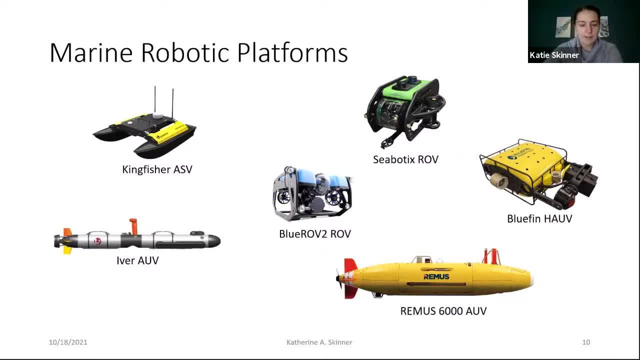 highly efficient applications. So these robots, from the ROVs, which are tethered, remotely operated vehicles, to ASVs or autonomous surface vehicles, and the Iver autonomous underwater vehicle you saw in the video before, can carry out very safe, efficient and systematic surveys over large areas. So these surveys can provide us with 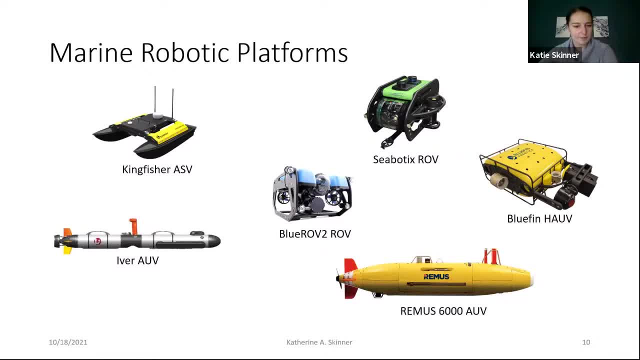 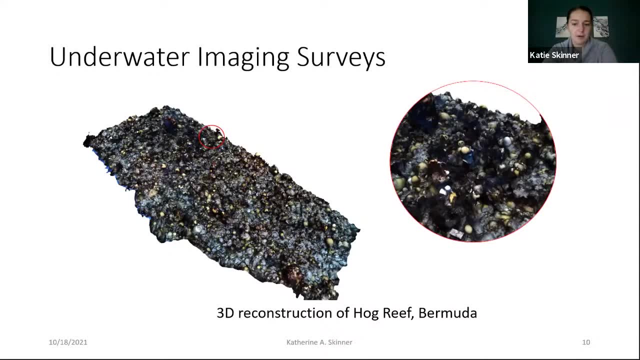 terabytes of image data and, using computer vision algorithms, we can create high resolution, colored 3D models of the seafloor with data collected from robots or automated imaging systems. So this is a 3D reconstruction created from imagery collected in Haagree, Bermuda, And the goal of this survey is to create high resolution 3D models of the seafloor. 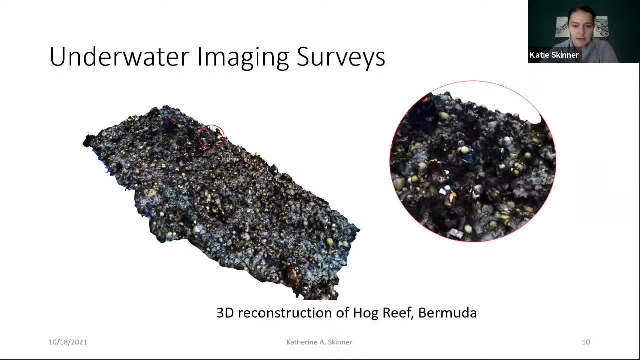 from imagery collected in Hog Reef, Bermuda, and the goal of this survey was to be able to identify scientific instruments placed throughout the reef structure and to be able to monitor this reef over time. So one thing to note here is that this reef reconstruction was created offline. 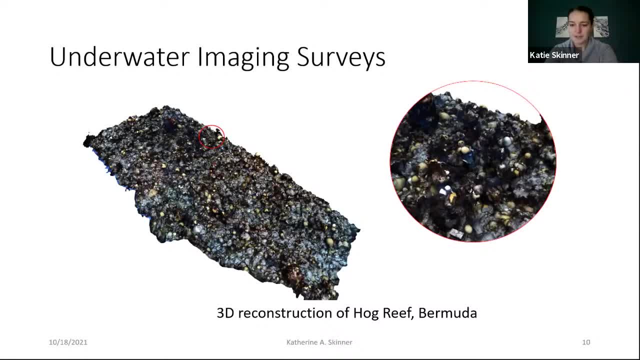 so, after we completed the survey, collected the imagery and compiled it. it still took several days to create this high resolution colored survey of the environment, and we really want to work towards being able to equip our robots and our autonomous vehicles with the ability to. 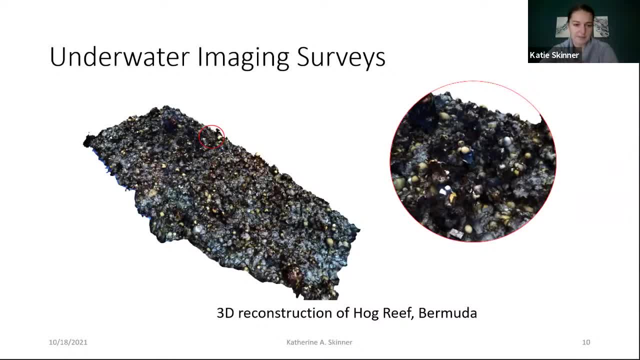 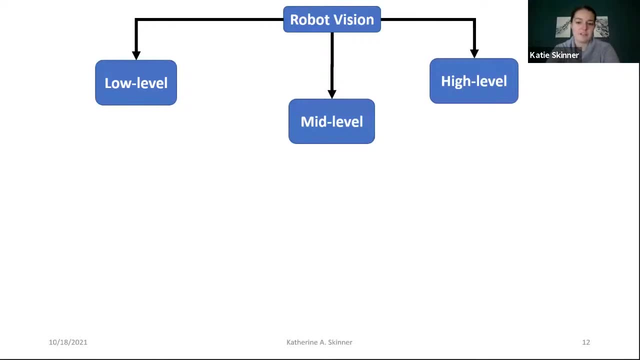 perceive a 3D environment on board the vehicle themselves and reason about different objects in that scene to better survey the underwater environments around us. I want to talk today about challenges across the span of robot vision and opportunities that we have to really overcome some of these challenges and push marine perception forward. 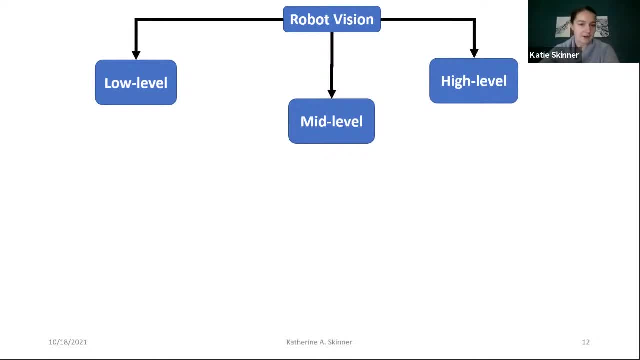 So I kind of map it out in terms of the hierarchy of vision which, like human vision, has low-level, mid-level and high-level components. So low-level vision really refers to taking the raw sensor data and processing it, perhaps to denoise. 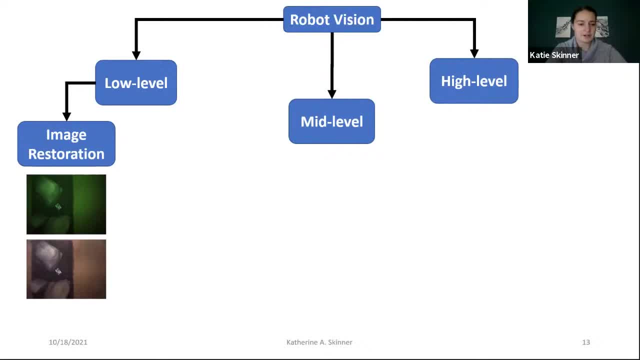 it or, in the case of underwater imaging, to perform image restoration, which I'll talk a bit more about what exactly that means. but this takes the raw sensor data and outputs it in a more usable format. In the mid-level range, we have tasks such as dense depth estimation. 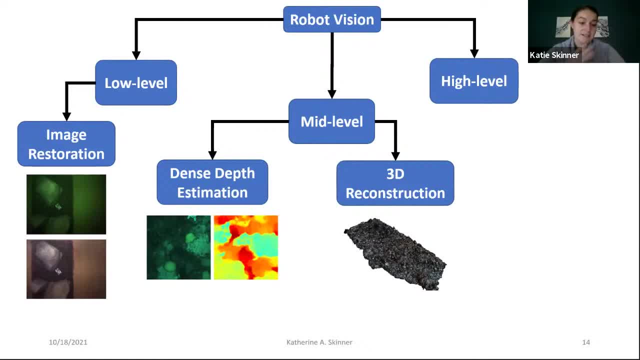 or 3D reconstruction, where we're taking now the processed sensor data and putting it into a different representation or a different format for some higher-level tasks, where higher-level tasks can really start to think about scene understanding. So that might include scene segmentation or object detection, but really a way to process the scene. 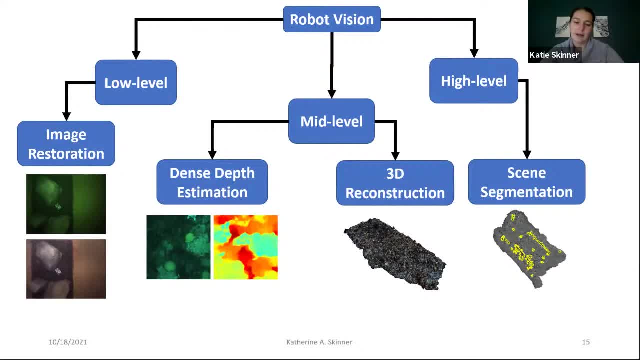 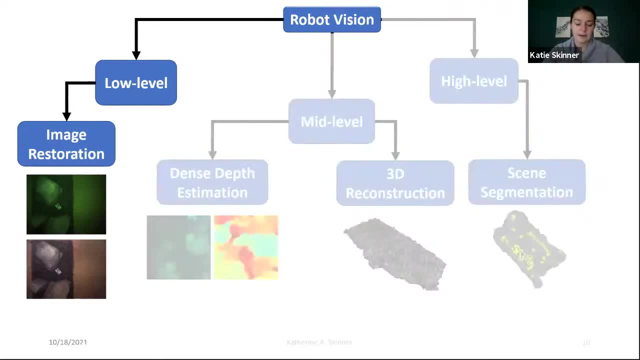 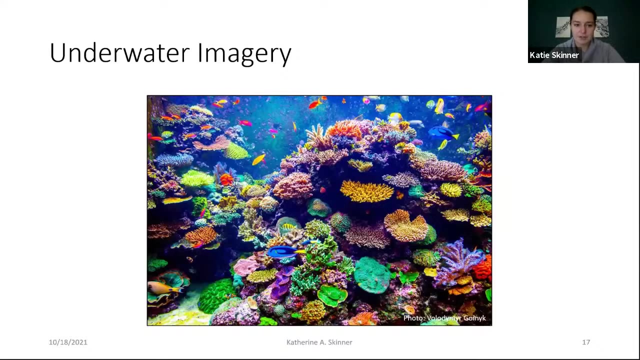 the full scene itself and draw out semantic information or higher-level information that scientists or other surveyors can use to make informed decisions in these environments. So first I'll start with talking about challenges and some methods I've developed To overcome challenges for low-level vision tasks like underwater image restoration. 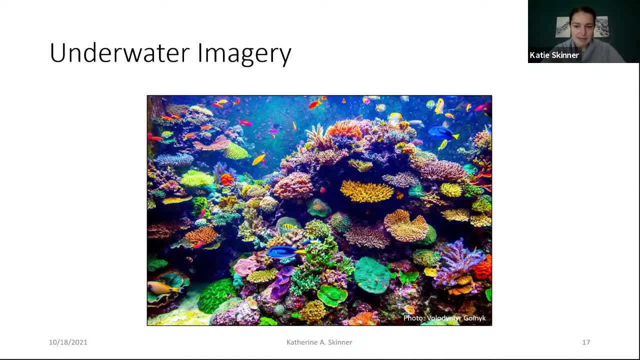 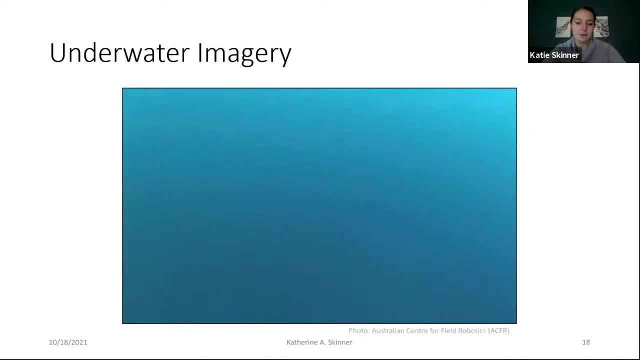 So when most people picture underwater imagery, this is what they see. They see clear water, brightly colored coral and fish, and unfortunately, these images are mostly thanks to Photoshop, And what we actually see when we look at our raw underwater images collected on board vehicles looks something more like this, So visibility can vary, of course, depending on 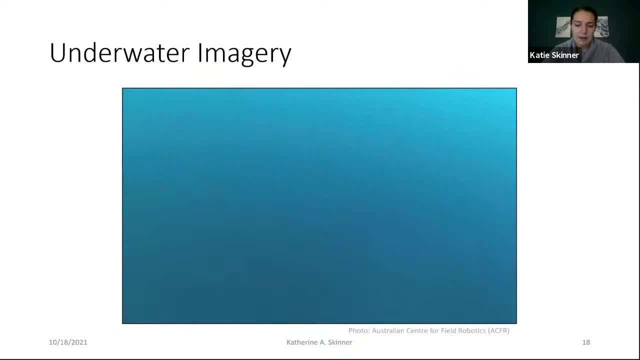 the underwater environment. You may get a clearer or hazier water, But typically for imaging surveys we consider surveying about two to four meters above the sea floor. So you can see as you get four meters, three meters, closer and closer, you can make out more features of the environment. 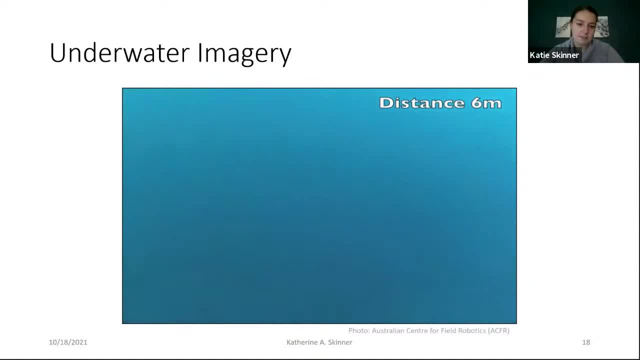 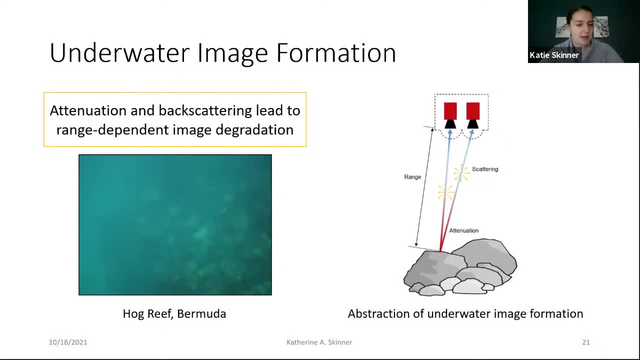 But we have a pretty constrained range that we can make out visible features in RGB imagery in underwater environments. look to physics-based models of underwater image formation or why this occurs. So, as a photon of light travels between the camera and the scene, it interacts with particulate matter in the water. 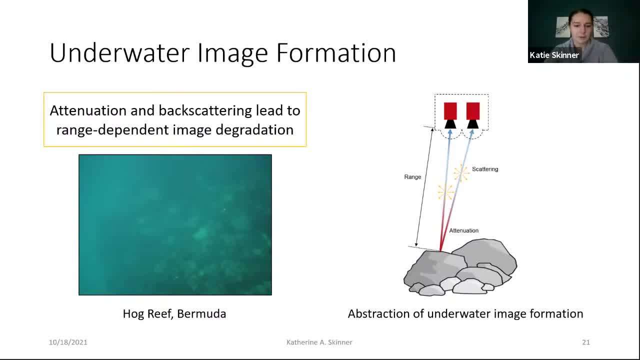 column and this can cause it to be scattered or absorbed. So absorption causes attenuation, which is wavelength and range dependent, and scattering leads to kind of a haze effect across the scene. But we can look to mathematical models for explaining some of these physics-based 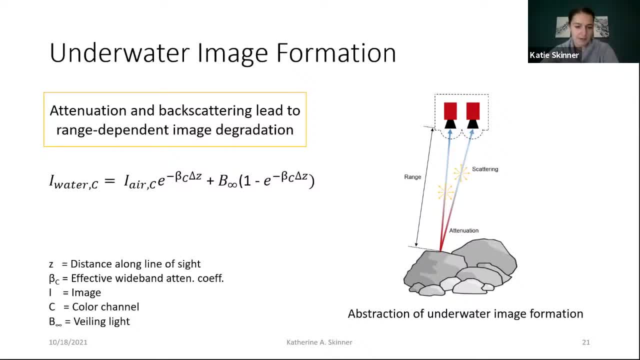 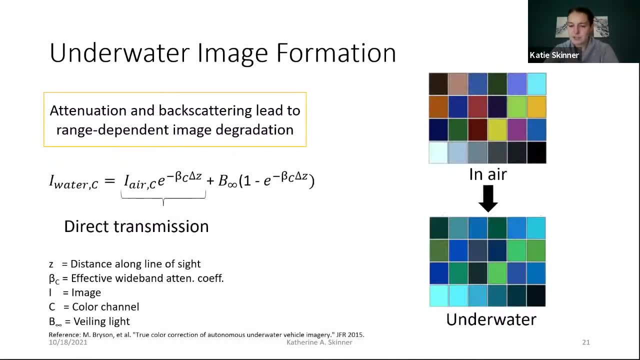 phenomena, So the process of underwater image formation. the model for underwater image formation contains two components. One is the direct transmission, which refers or which relates to this attenuation effect, where, if we were to look at colors imaged in air and then those same, 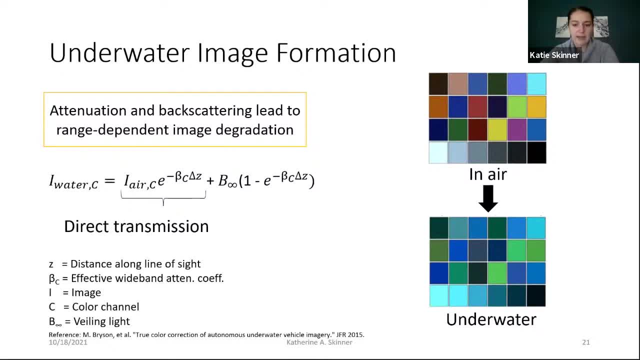 colors imaged underwater, we would see this exponential decaying. So if we were to look at the decay of colors for RGB cameras, it occurs at different rates for different wavelengths, with ocean environments showing a higher rate of attenuation for the red channel specifically. So this might be a color board imaged in an ocean environment. 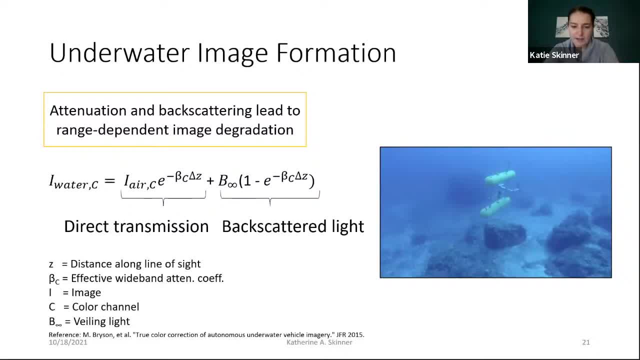 And the second component is kind of this added component of backscattered light And you can see that this occurs kind of similar to a fog effect in air. If you were to think about viewing a foggy scene, you would see this kind of effect in the air. So if you were to look at 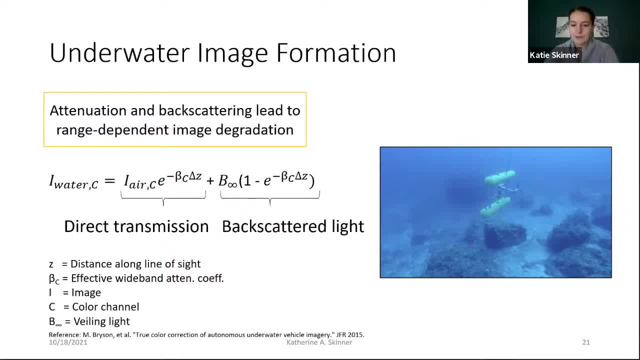 a scene you can see. as you get further and further away from the camera, you see this haze effect that really degrades the image from how it would appear if just imaged on land. So what's important to note is that these underwater effects are range dependent. 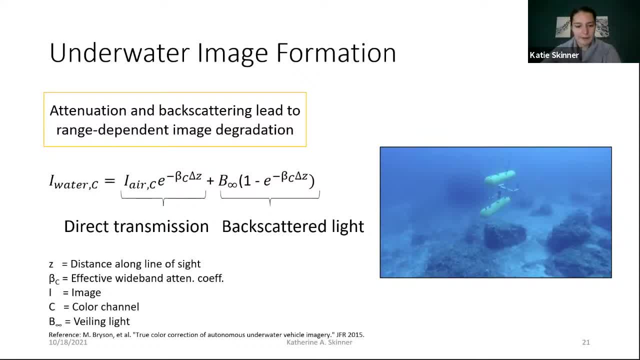 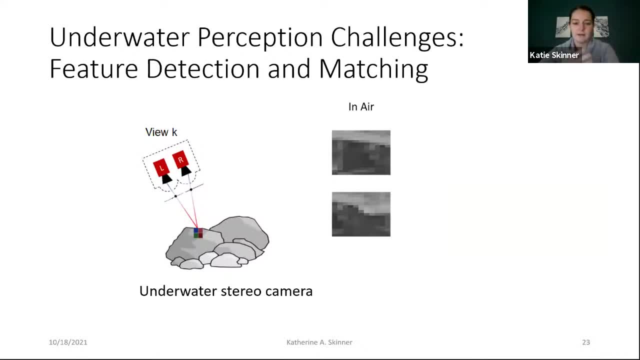 So they depend on the distance along the line of sight, And this range dependency has a couple of really important consequences for underwater perception and computer vision. So one challenge that this raises is that for images in air, when we thought of developing feature detection matching algorithms in traditional computer vision approaches. 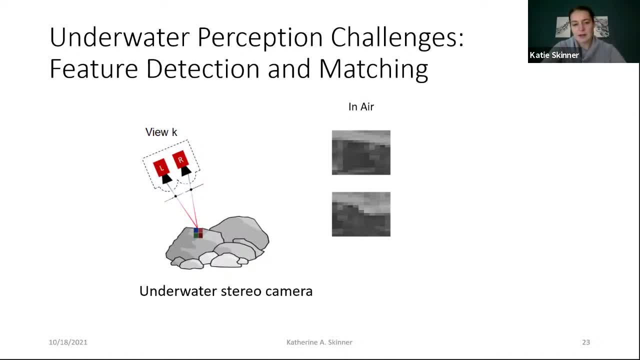 we typically rely on ideas such as contrast to make sure that we are detecting repeatable and reliable features and imagery And, unfortunately, due to these underwater effects, the same image patch will not be able to detect these underwater effects, So we're going to have to look at the 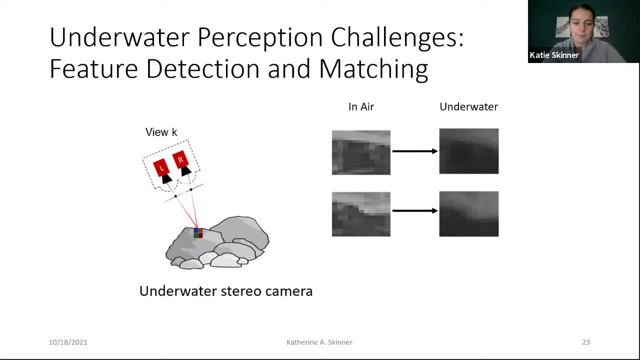 same patch on an object, So this was on a rock platform imaged in air. If we were to image this same feature underwater, we see much reduced contrast in the image patch itself. So this really raises a challenge in transferring methods that we've developed on land, especially for 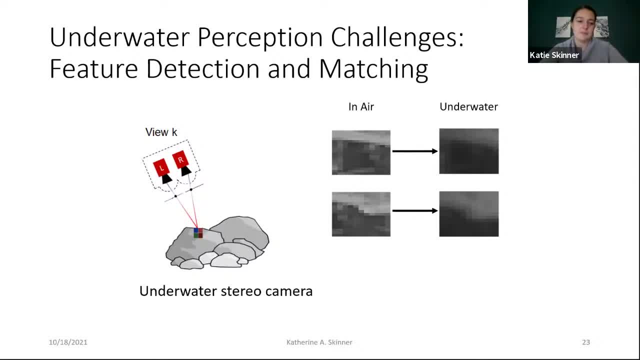 feature detection To be able to transfer those methods underwater. we typically need to do some sort of processing in order to leverage those. So this is a challenge that we've developed on land, especially for feature detection to be able to transfer those methods underwater. We typically need to do some sort of processing in order to leverage those methods. 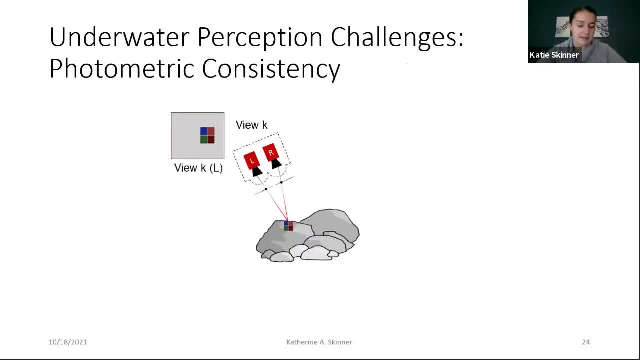 The other challenge that this raises is challenging photometric consistency. So on land, especially with the popularity of direct SLAM methods in recent years, we use this constraint that we assume that if we view a feature point from one angle and one viewpoint and then we move to a different viewpoint, we'll have some measure of 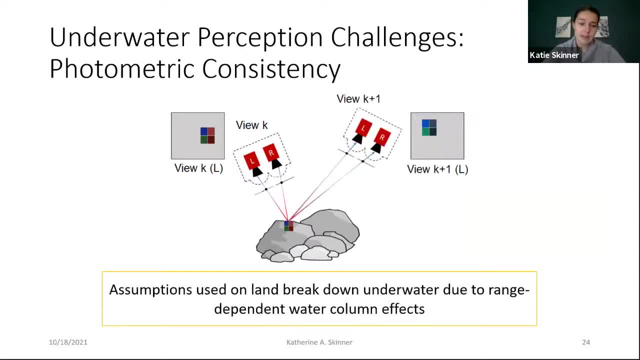 brightness constancy or photometric consistency And unfortunately, when we look at these cases underwater, we see that these assumptions can break down due to the range-dependent effects. So since attenuation and backscattering are range-dependent, if we move to a different perspective, that's, at a different range, we can see inconsistent. 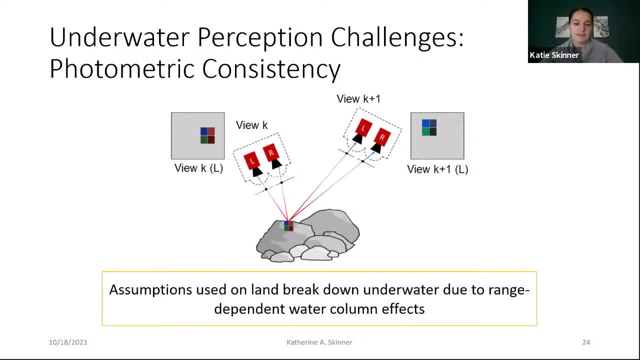 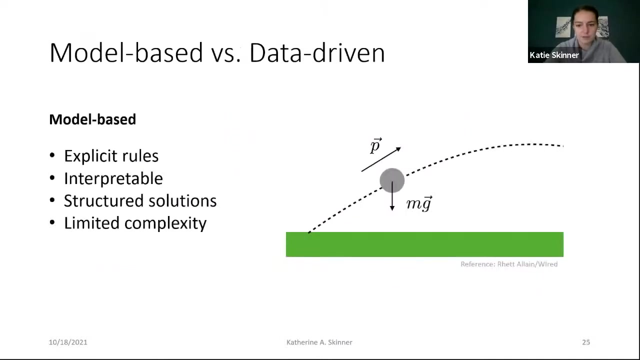 intensities and colors across these ranges. So this is really a challenge for leveraging SLAM and computer vision methods that have been developed on land for terrestrial applications directly to underwater environments. So the first challenge I want to focus on is how we can address these issues related to water column effects. 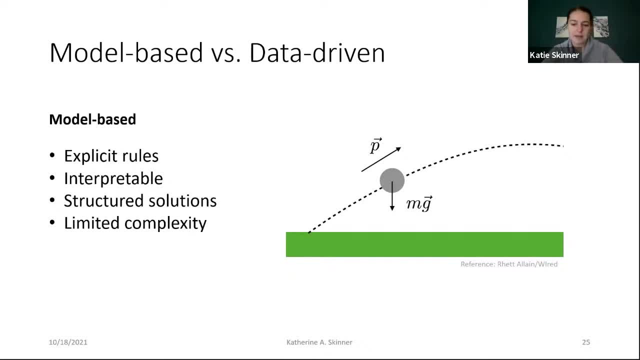 And many people have come up with ways to think about these problems. So there are kind of two approaches. The first is a model-based approach. So looking at the physics-based model of underwater environments, we can see that the water column effects are very different from 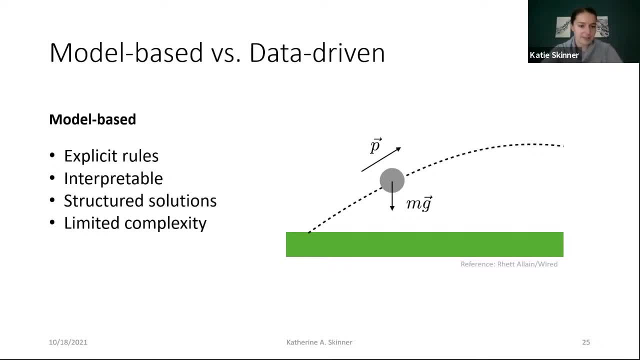 the underwater environment. So we can see that the water column effects are very different from the formation or physics-based models. in general, We tend to have explicit rules that are interpretable and provide more structured solutions to what we are trying to solve, But unfortunately, 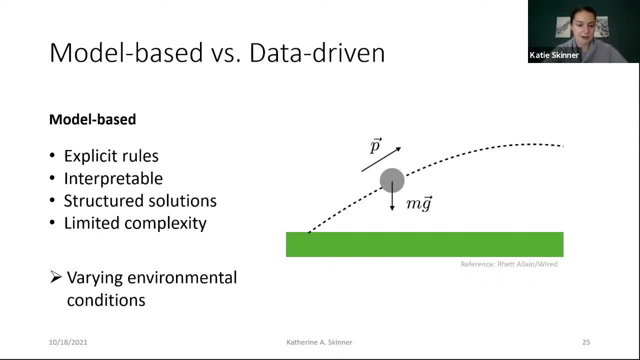 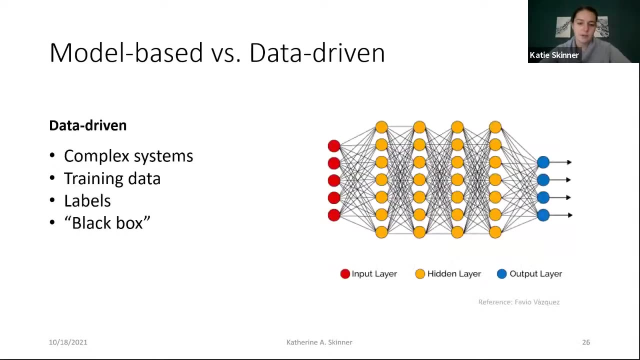 it's difficult to model every effect that might be occurring. So if we have varying environmental conditions, as we do underwater, it can be challenging to find a solution for modeling every single water column effect that we might see or encounter. Alternatively, you can take a data-driven approach, such as machine learning or 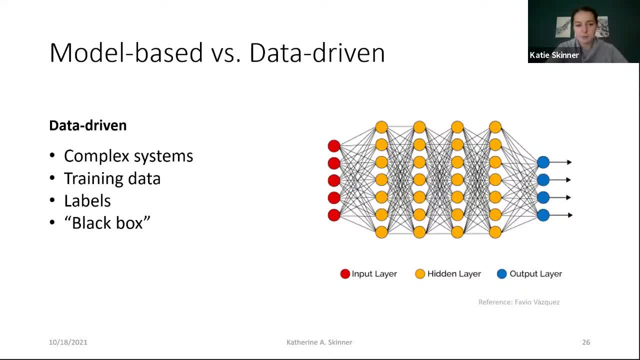 deep learning approach And data-driven approaches are capable of modeling very complex systems using training data that contains some input and, typically for supervised learning, labeled output as well, And data-driven approaches can then model very complex processes, but unfortunately they're referred to as black boxes, And so we can model very complex processes. 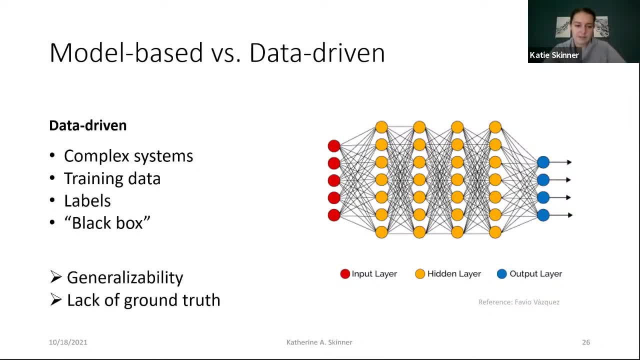 that contain some input and typically for supervised learning, And so we can model very complex processes. but unfortunately they're referred to as black boxes, And so we can model very complex processes And there are challenges to generalizability across different environments And what's a major 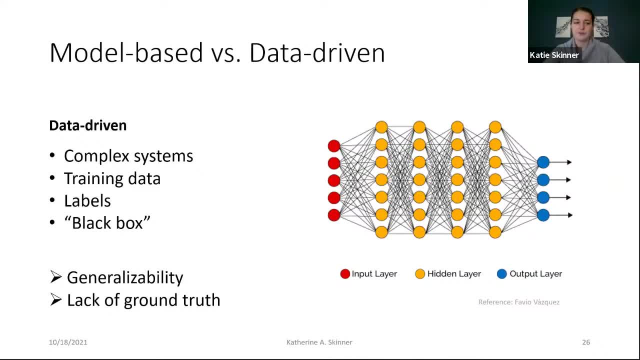 challenge for underwater perception is that we have a lack of ground truth for many tasks that we would want to perform. So if you think of the challenge of underwater image restoration, we don't necessarily have ground truth for underwater color of every scene that we might. 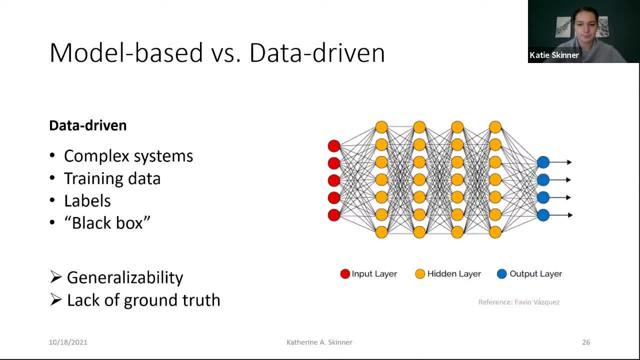 want to process, And so we can model very complex processes that we might want to perform. So kind of the opportunity we have here is: we've had success in both of these areas and is there a way to leverage success of both model-based and data-driven solutions? 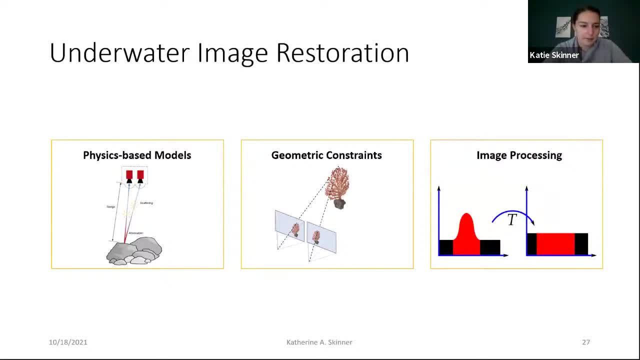 So I've worked on problems to basically integrate physics-based models into deep learning frameworks, as well as other constraints such as geometric constraints about the sensor configuration or ideas from image processing, to allow us to structure deep learning frameworks in a way that can overcome this lack of ground truth. 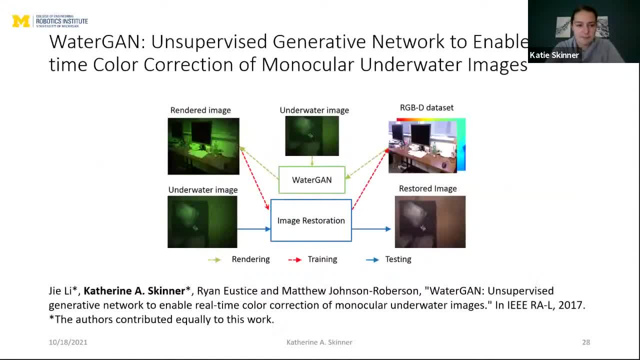 So I'll focus on one method where we integrated physics-based models into a deep learning framework for performing underwater image restoration, And this work was called WaterGAN. So it is an unsupervised generative network for color correction of monocular underwater images. 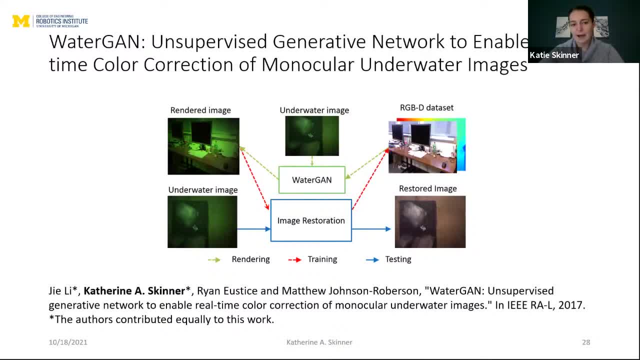 And this network works without having to have any ground truth, color or depth of underwater scenes that you are working with. So the first step is to generate synthetic underwater imagery, So taking RGB-D data collected in air and transferring this to have realistic underwater effects of the underwater environment that you are seeking to restore. 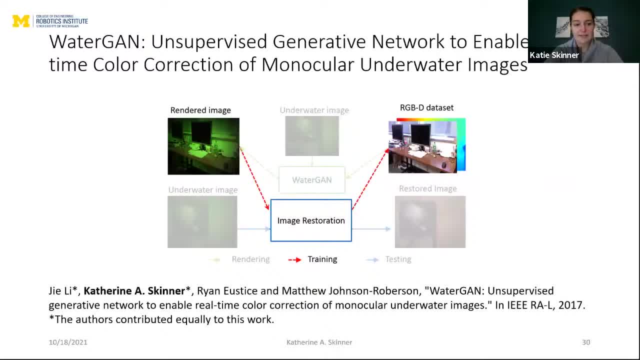 Then we train an image restoration network that takes in this synthetic underwater image and outputs the ground truth in air, RGB color and the depth map of the scene, And then, lastly, during test time, we can take just the monocular underwater image as input. 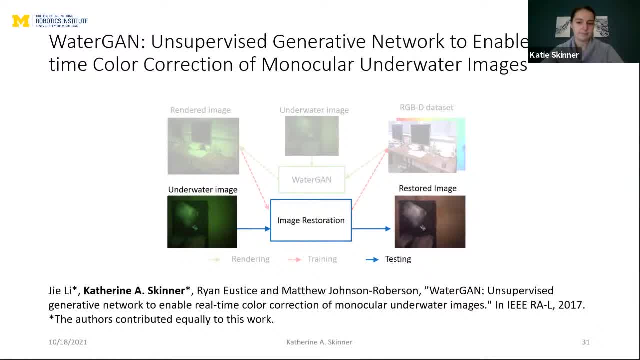 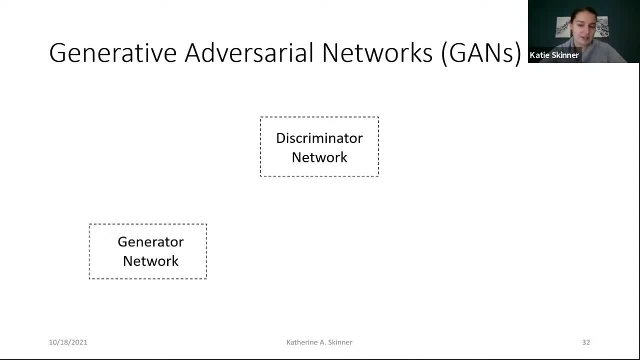 and output a restored image of that underwater scene. So I'll walk through a little bit more about how this network incorporates the physics-based model of underwater image restoration. But first just an overview of generative adversarial networks which form the backbone of the WaterGAN network. 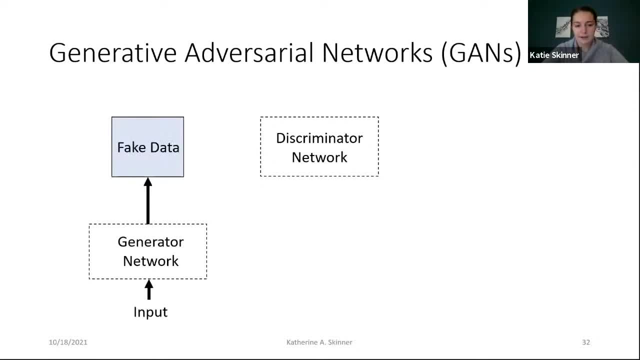 So GANs have two networks that are kind of competing: the generator network and discriminator network. The generator network takes some input and outputs fake or synthetic data And then the discriminator network sees the fake data and the real data and needs to determine whether that data is real or fake. 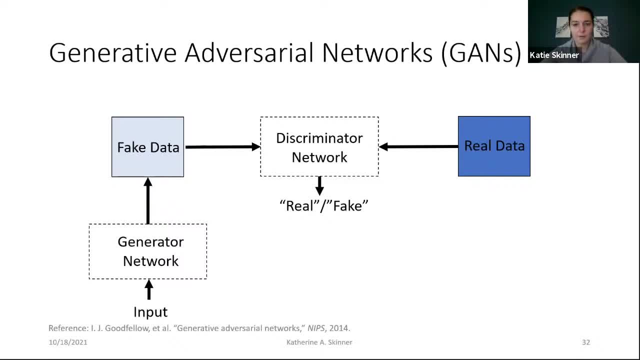 So, since we know what data comes from the generator network, we know which data is fake. So in this way, we get our labels for free And the generator sees the output of the discriminator network, so it can constantly try to improve its fake data generation process in order to fool the discriminator network. 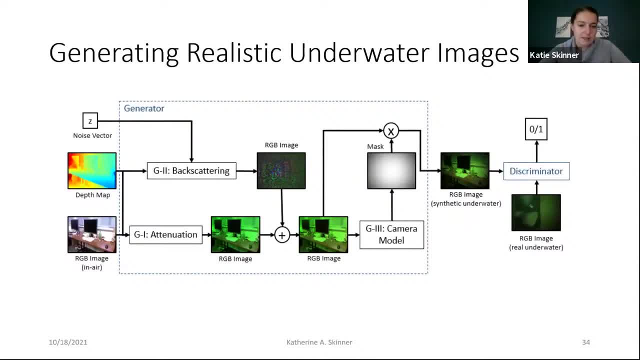 So this is the overview of the WaterGAN network. So the WaterGAN network features a generator that's really inspired by the process of underwater image formation. to add structure for training For this problem, the generator network takes in a RGB image and a depth map. 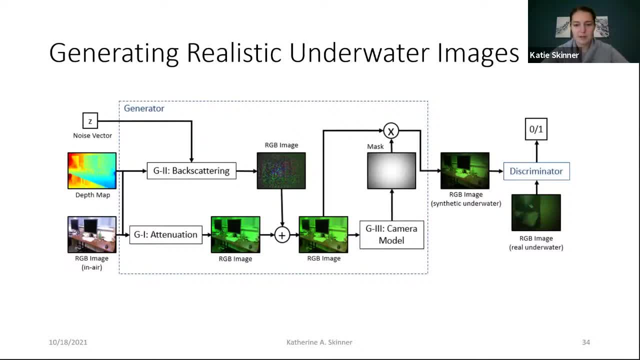 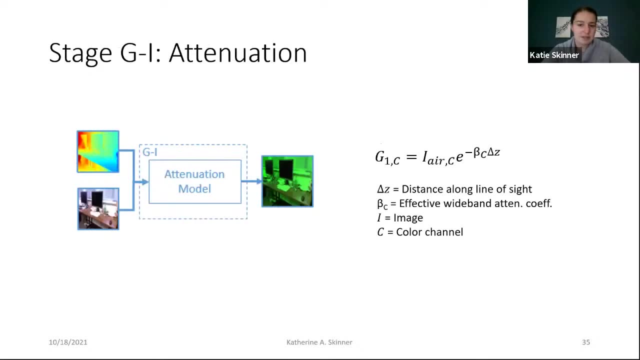 So this was collected from open source RBGD data sets, as well as the noise vector, And it outputs a synthetic underwater image that matches the distribution of underwater effects seen in a real underwater data set. There are three stages in the generator network, So the first is modeled after attenuation. 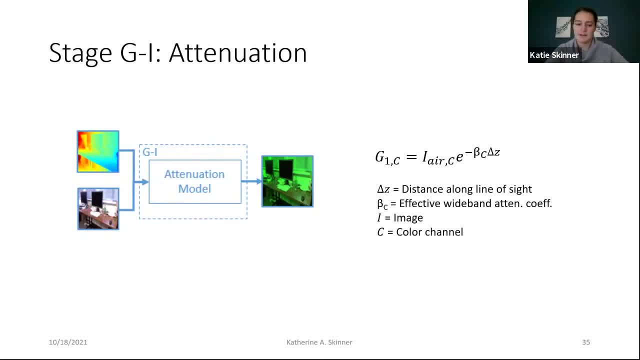 So, based on the physics-based model of attenuation, we are seeking to learn simply the attenuation parameters for this underwater environment. So for RGB images we have one parameter for each color channel, So we have the attenuation of red, green and blue channels. 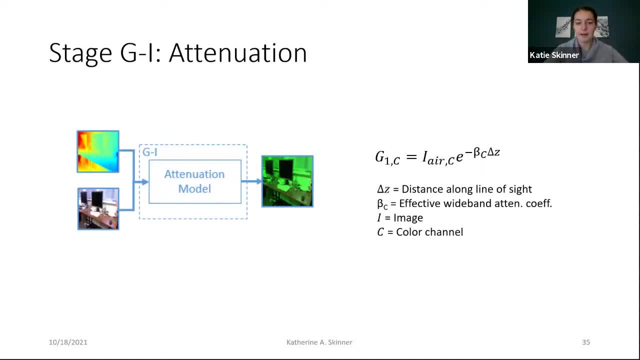 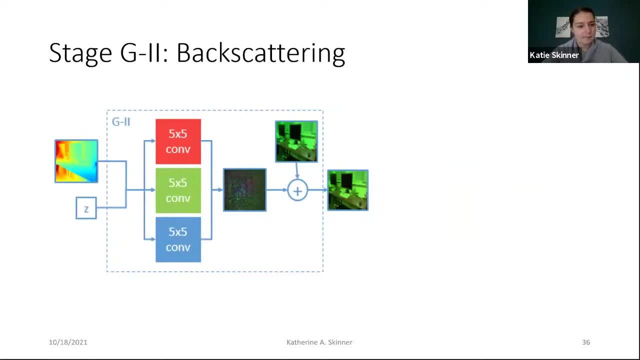 So the attenuation model is simplified by incorporating knowledge of the physics-based model of underwater image formation, And then we have a backscattering module that adds on a mask, similar to how backscattering occurs in the physics-based model. Here we learn the mask and then it gets added to the attenuated image. 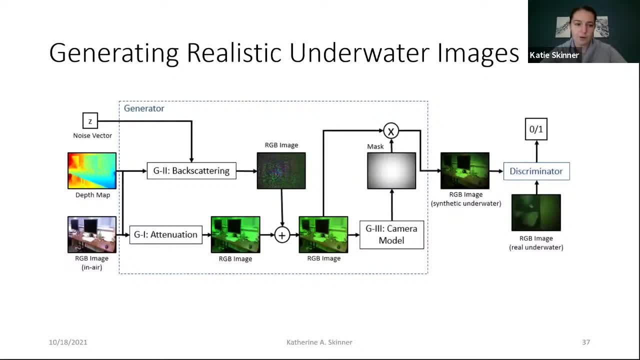 And we also modeled camera models for modeling vignetting effects, since that was important for this data set specifically. So at the end of this process, WaterGAN outputs a synthetic underwater image that is now aligned to a ground truth RGB image and depth map. 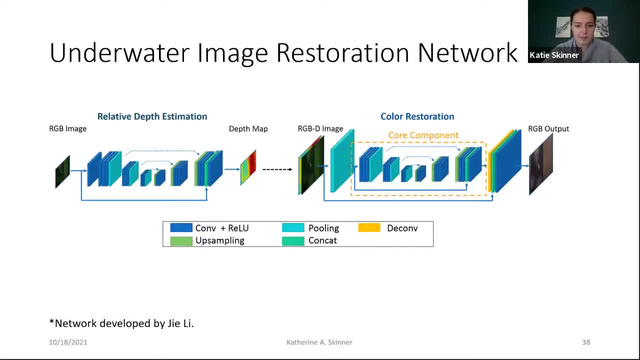 Next, we can train using this synthetic data. we can train an underwater image restoration network to go from that synthetic underwater image to a depth map. And since we know that the image restoration is range dependent, we can patinate the depth map to that RGB image to learn the final output for the restored image. 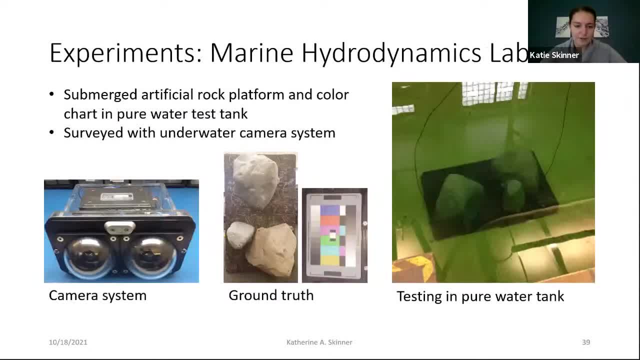 And, of course, as I mentioned, it's very difficult to get ground truth underwater. So we create our own synthetic platforms, artificial rock platforms, in order to perform experiments, to make sure that we can evaluate our methods quantitatively and qualitatively. 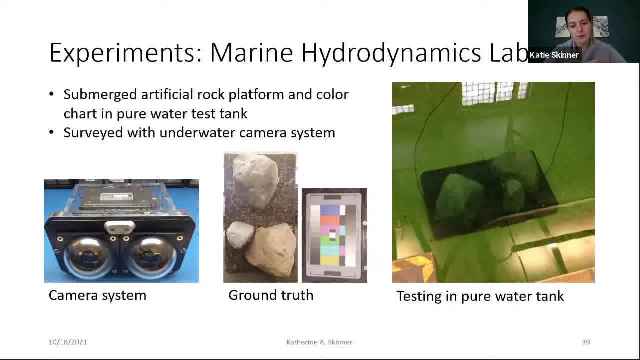 So this is a submerged artificial rock platform that we submerged in the water tank And we surveyed this platform with a stereo camera system And we also we also can submerge a ground truth color board to give us ground truth colors only for evaluation purposes as well. 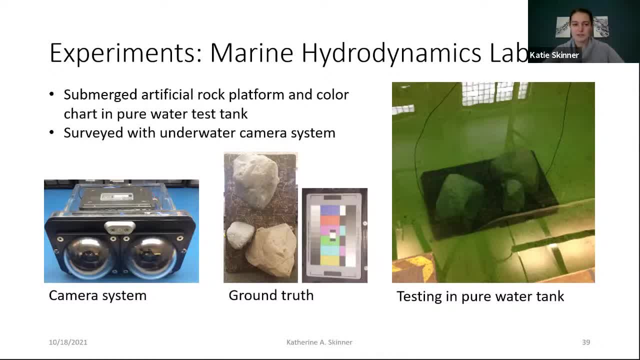 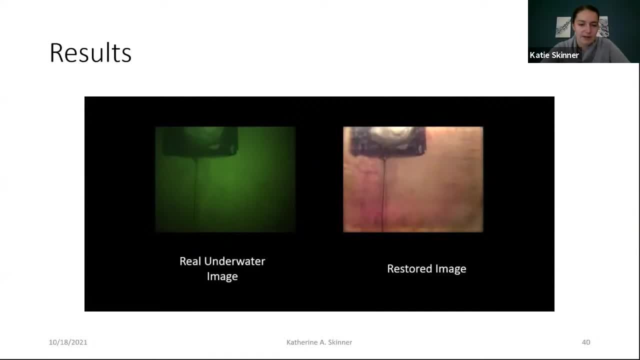 So when we train the WaterGAN network and the image restoration network, this is the output that we see. So for the real underwater image on the left, that is the input during test time and the output is the restored underwater image. So this shows kind of the quality that we're able to achieve. 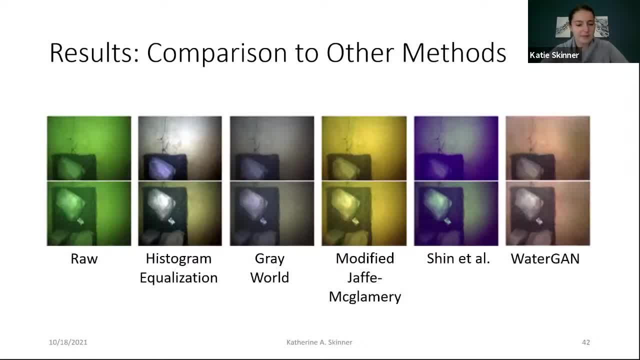 without having any ground truth, color or depth of underwater imagery for training or as input for testing. And we're of course interested in the accuracy of the color reconstruction. So we can use the color board to determine quantitative evaluation for accuracy of restored colors. But we're also interested in restoring this assumption of photometric consistency. 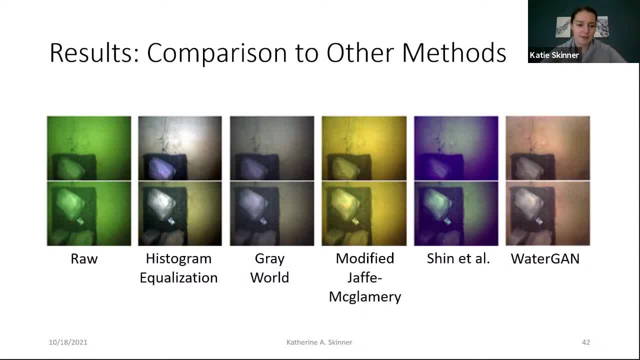 So we're interested in seeing consistent restoration across different methods or across different viewpoints. So we compared to several different methods. Specifically, the histogram, equalization and gray world methods are image processing approaches, So these most methods don't have any knowledge of the physics based model of underwater image formation. 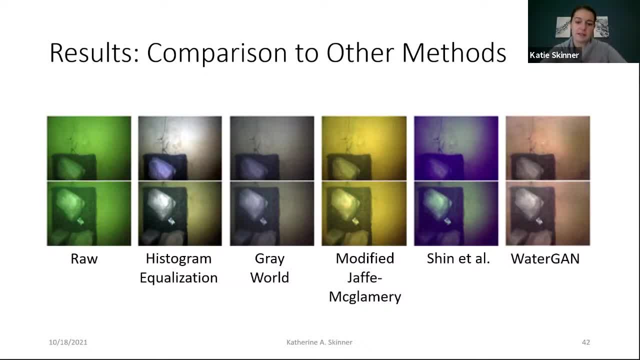 They're not incorporating any notion of range dependency in the restoration process, So you can see that these methods can give sometimes inconsistent restoration results, Whereas our method is able to provide consistent color correction across viewpoints from different scenes. One thing we were interested in seeing is if we could learn monocular depth maps. 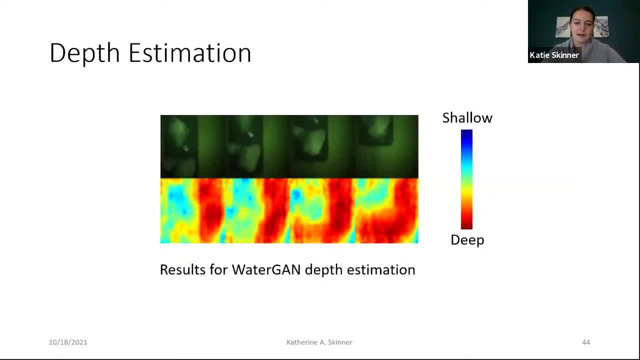 or monocular depth reconstruction from this method And we found that we could determine accurate relative depth for our underwater images. But they weren't accurate absolute depth estimates. But this is one area that I think would be a really interesting opportunity, since the process of underwater image formation is depth dependent. 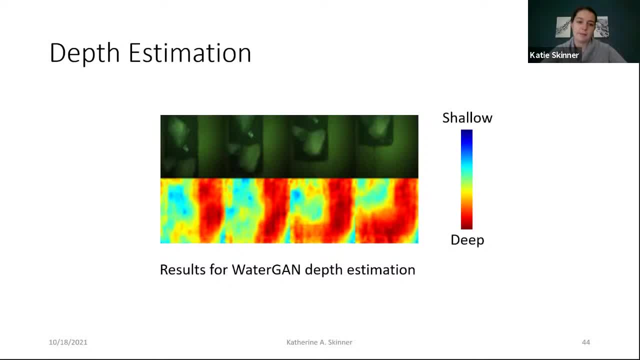 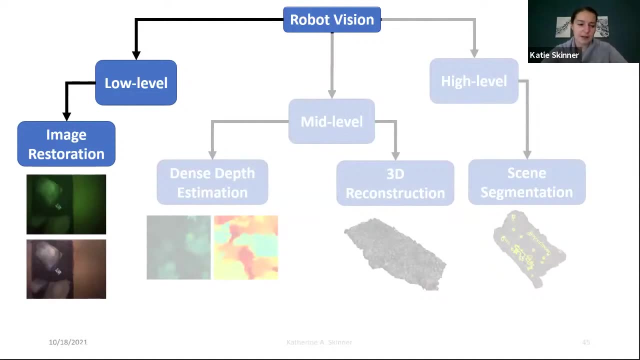 that you should have some extra information on top of what you have in terrestrial scenes to perform monocular depth estimation from underwater imagery. So this is kind of the low-level imaging challenges and how we can use deep learning, specifically by integrating knowledge of model-based solutions for performing image restoration. 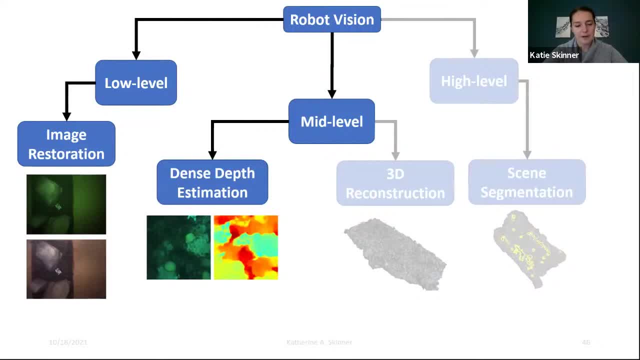 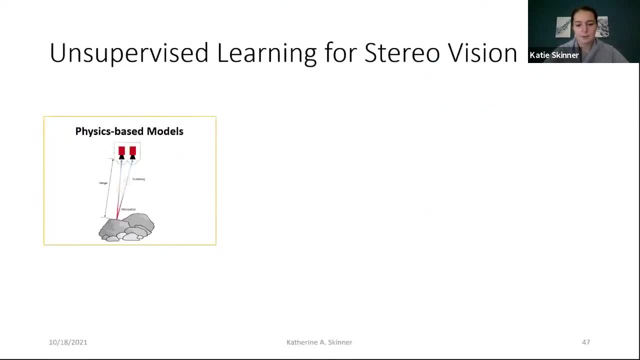 So I want to talk about how we can incorporate other constraints as well, that we might have known from our sensor configuration on our robot platform or from the image processing community as well. So for this work we extended to stereo vision to enable unsupervised learning. 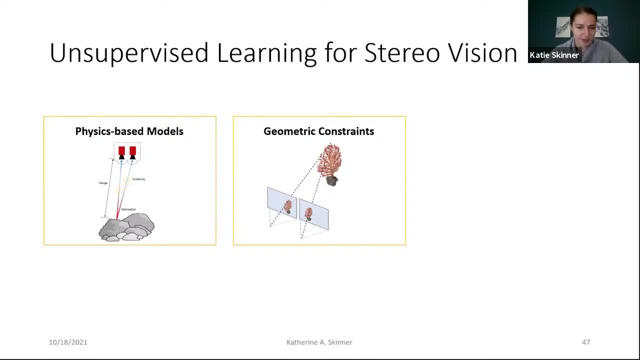 for image restoration and depth map estimation from underwater stereo images. And again, our goal was to do this without having ground truth, depth or color of our underwater scene. So we incorporated physics-based models or ideas from physics-based models, again, as well as geometric constraints from the stereo vision configuration. 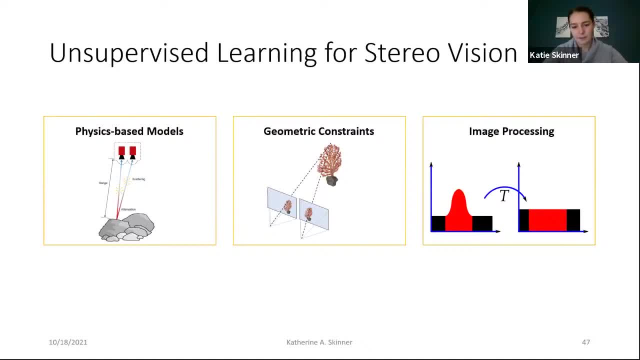 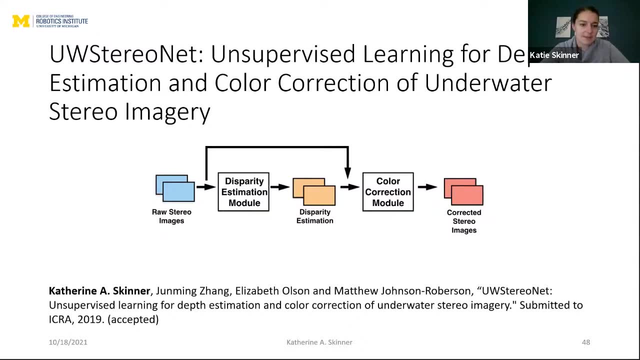 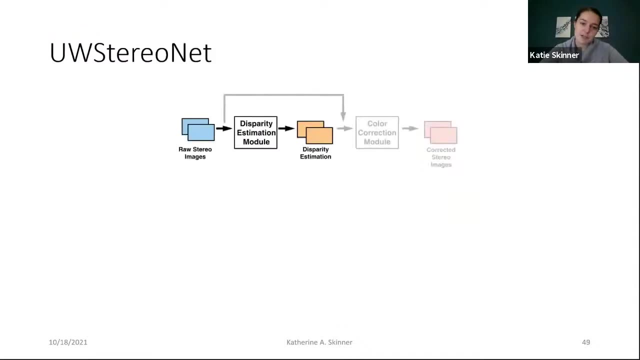 and image processing approaches, And this work was called Underwater StereoNet, which is unsupervised learning for depth estimation and color correction of underwater stereo imagery. So again, this network had two modules, So the first module was focused only on disparity estimation. 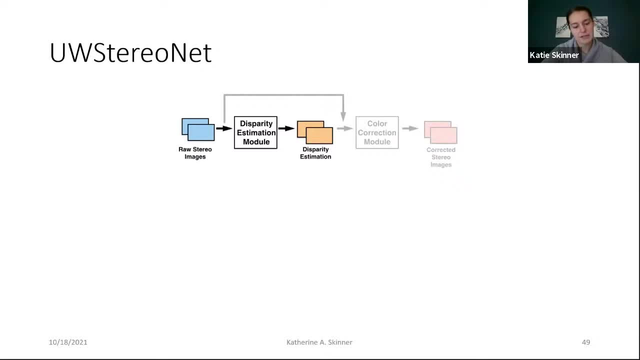 where it took input raw underwater stereo images and output disparity map, And here we really leveraged geometric constraints to learn left-right consistency of the output depth map. And then the color correction model took input raw images and these estimated depth maps to output the corrected stereo images. 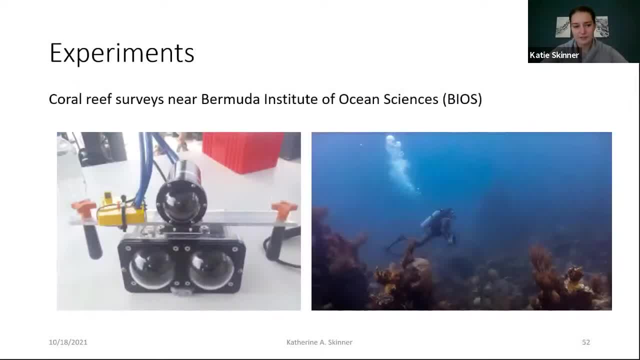 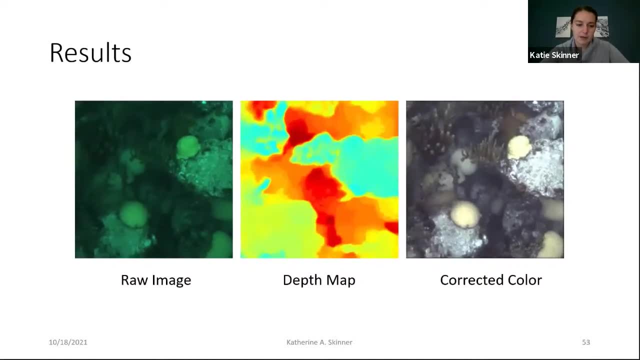 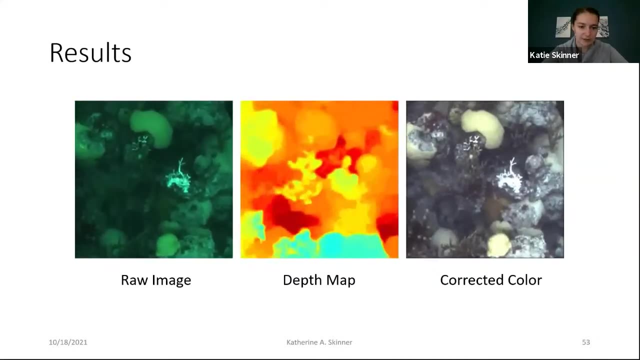 And we performed some experiments in coral reef surveys. So this was again near hog reef, Bermuda, with a stereo diver rig to collect data, And I'm only showing one image of the stereo pair here, but we have the input raw image, I think the left image on the left. 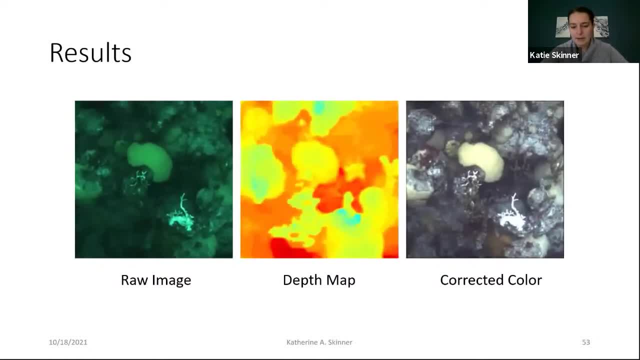 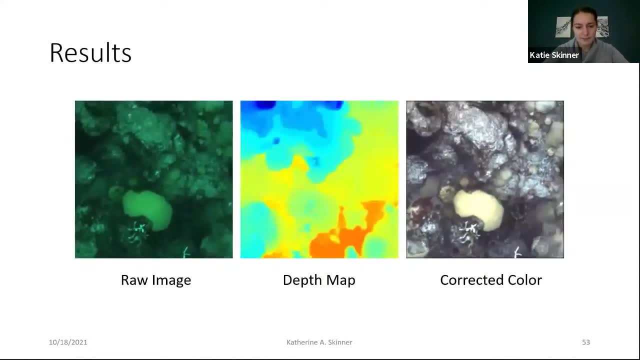 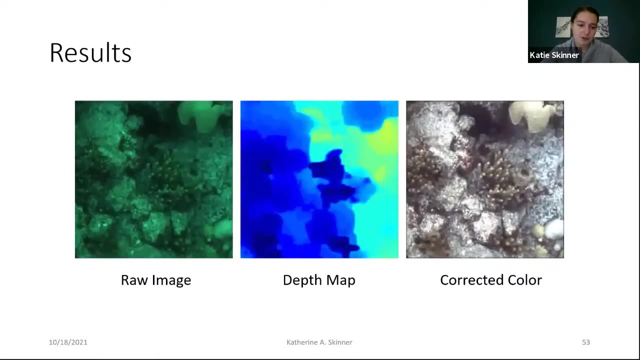 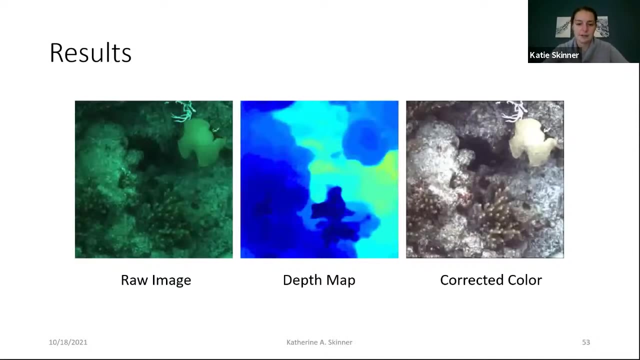 And the output of our method is now a dense depth map and the corrected color image from this raw input underwater image. So again, this output- depth map and corrected color- are enabled without having any ground truth color or ground truth depth of underwater scenes, And this is really this unsupervised approach- is really enabled by incorporating constraints. 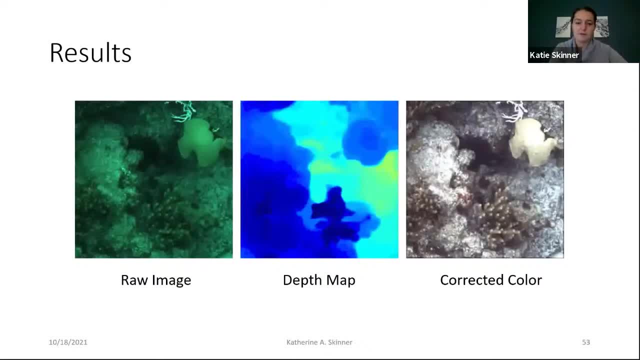 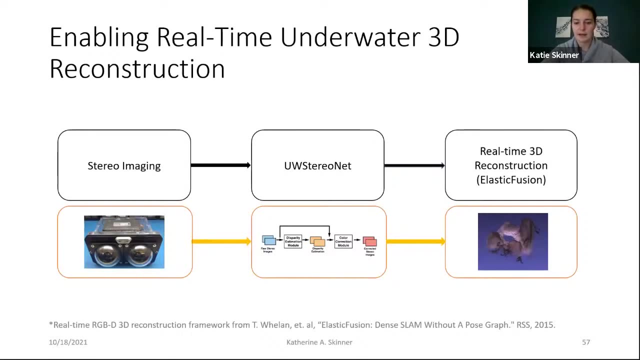 that we have from knowledge of the physics based models, as well as constraints from geometry and and knowledge from the image processing community as well. So we wanted to see how we could use this pipeline in an application for real time 3D reconstruction of underwater scenes. 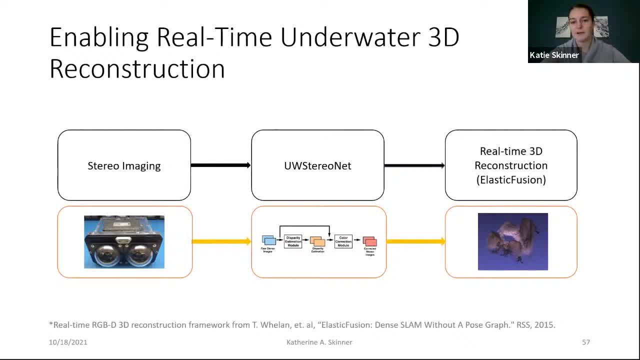 So, as I mentioned, we have the ability to create really high resolution colored 3D models of underwater scenes, but typically these are processed offline and can take several days and some human oversight to output an accurate 3D model. So we wanted to look at whether we could. 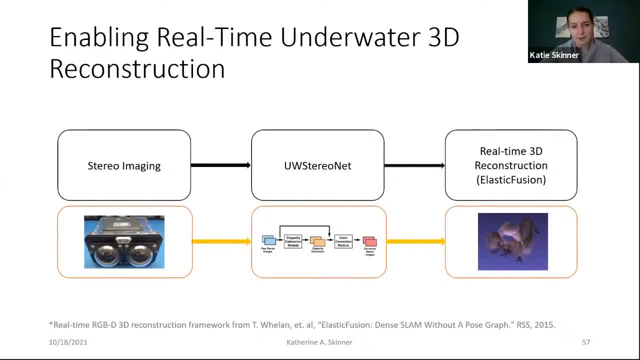 enable use this deep learning pipeline to enable real time underwater 3D reconstruction. So this framework takes in raw stereo images. It inputs those raw underwater images to underwater stereo net which outputs the RGB image and the depth map. We have the output at about two frames per second. 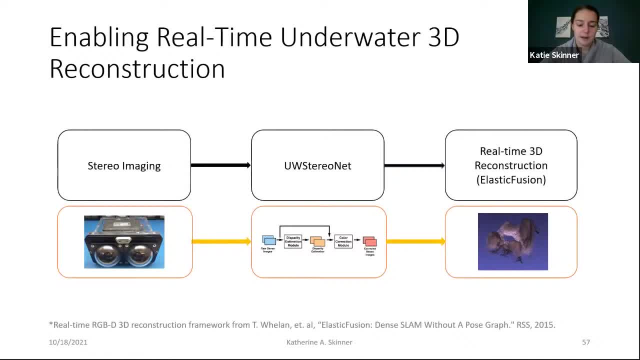 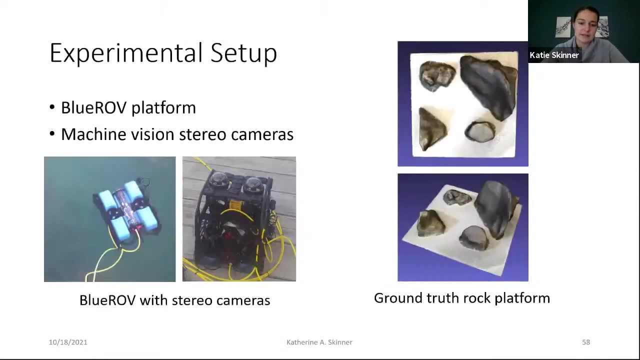 For purposes of this experiment, we were working with a laptop and streaming images over. So after we have images recorded on the laptop and we input the depth and corrective color images into a pipeline for real time 3D reconstruction. In this case, we used Elastic Fusion, which takes in RGBD data to output a dense 3D reconstruction. 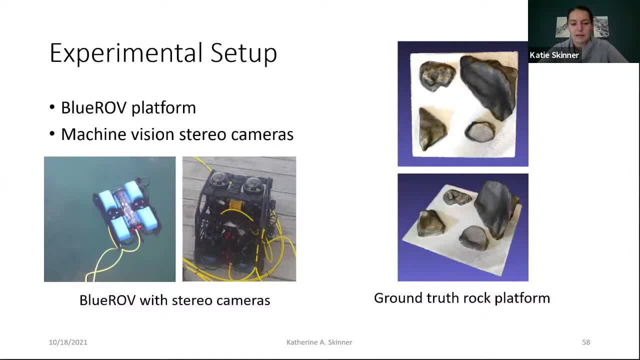 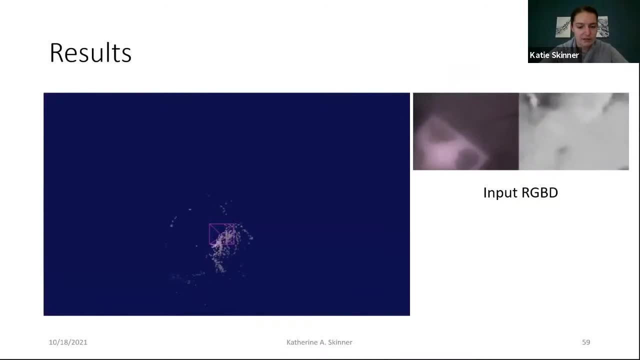 So our experimental setup was stereo cameras mounted on board a blue ROV platform And again we submerged over it. We used a rock, a artificial rock platform, to have ground truth for studying this problem. So this is the input RGBD which was output from our underwater stereo network and input to the Elastic Fusion pipeline. 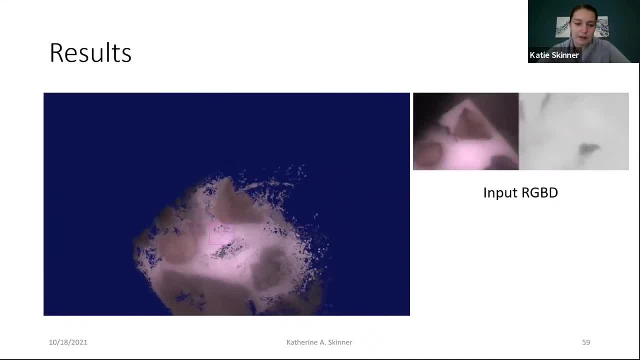 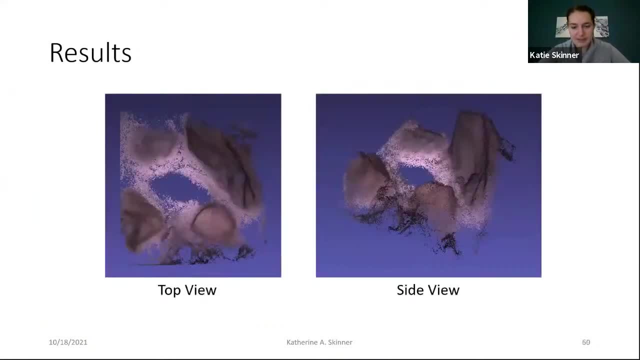 to perform real time 3D reconstruction of this underwater platform. So pretty promising results for this, which was exciting to see that we can kind of leverage deep learning pipelines to enable real time, real time 3D reconstruction and perhaps other processing for real time perception in underwater environments. 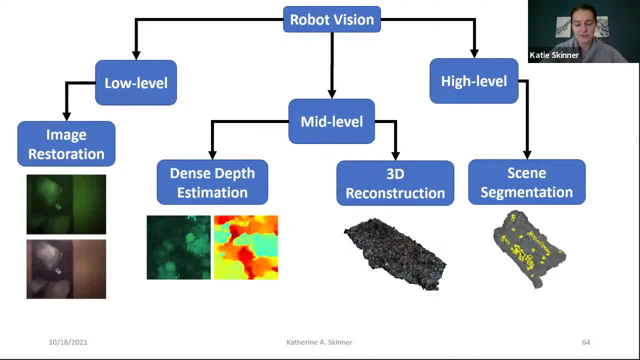 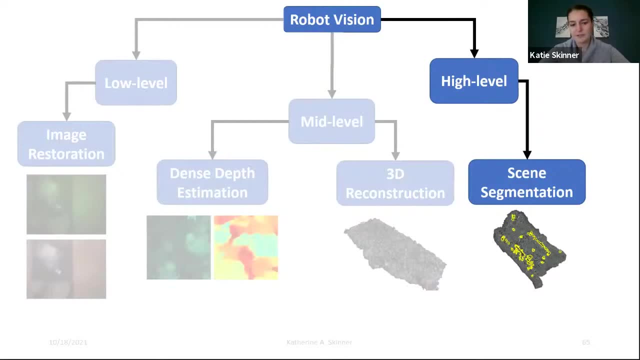 So this brings us to high level vision for scene segmentation, And here I just want to highlight some ongoing work that we have, that we have recently started in the field robotics group. So scene segmentation refers to the ability to process underwater imagery, process raw imagery. 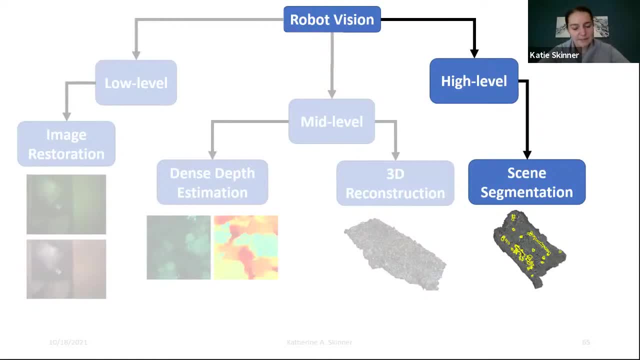 perhaps represented as dense depth estimates or 3D reconstructions and output some higher level knowledge of the scene. So this: in this case, here we were looking at a submerged underwater city where we wanted to detect manmade structure from the underwater underwater seabed environment. 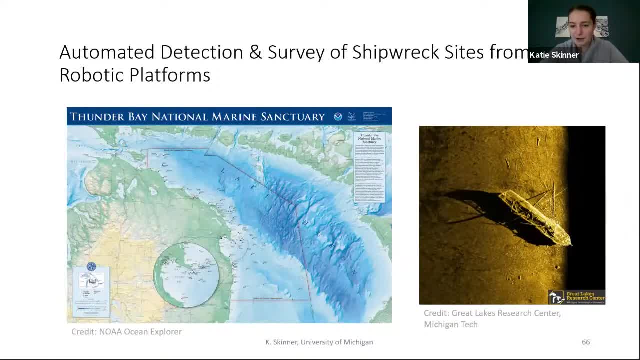 So in the field robotics group we have recently started a project for automated detection of shipwreck sites from our robotic platform. So this brings up a lot of the challenges of working in underwater environments that we have limited access to ground truth data for. 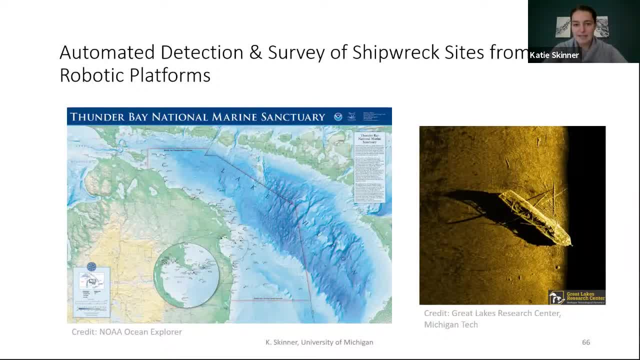 or label data, I should say for many tasks that we might want to pursue across marine robotics applications. So for this case, we're focused on working with side scan sonar data collected from autonomous underwater vehicles And we're going to be performing surveys and tests in the Thunder Bay National Marine Sanctuary. 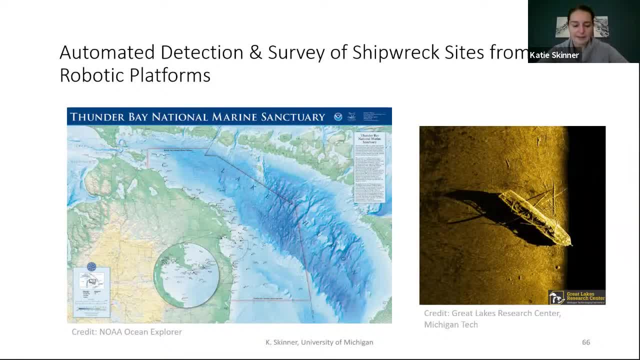 And the National Marine Sanctuary Thunder Bay is unique in its abundance of shipwrecks. So there are hundreds of known or unknown, but yet to be found shipwrecks that lie in Lake Huron, And we're going to really take advantage of this. 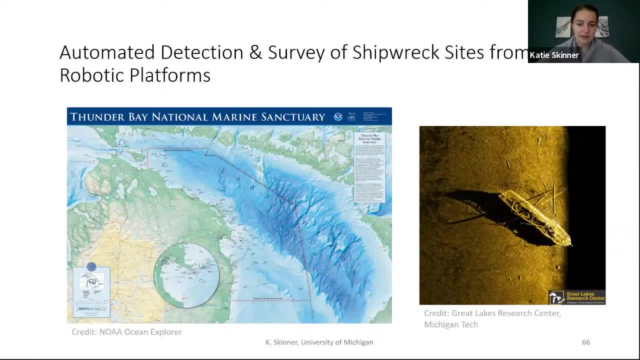 of this environment in order to collect really interesting data set of side scan sonar imagery for shipwreck sites And we're focused on the challenge of enabling automated detection on board an AUV of interesting of sites of interest so that we can survey these sites at a closer range. 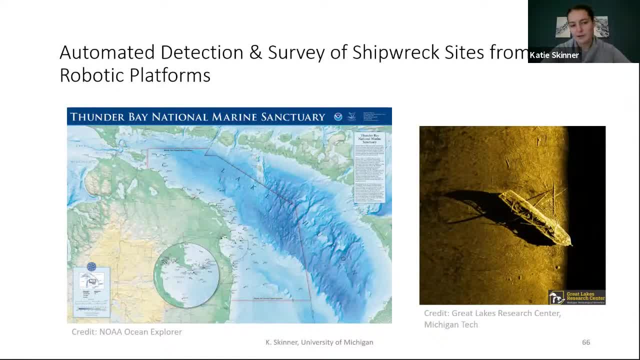 And there are many challenges to this problem, including lack of labeled data, but also just the challenge of processing a unique sensing modality for underwater vehicles. So we have some upcoming fieldwork for this project next year that we're really excited to get to get started on. 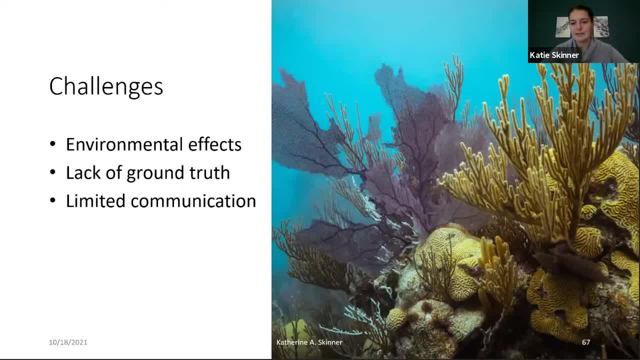 So I just want to kind of take the last few minutes to summarize the challenges that we have for underwater robot perception And, of course, one of the main challenges arises from the environmental effects, or these water column effects, that are really unique to underwater environments. 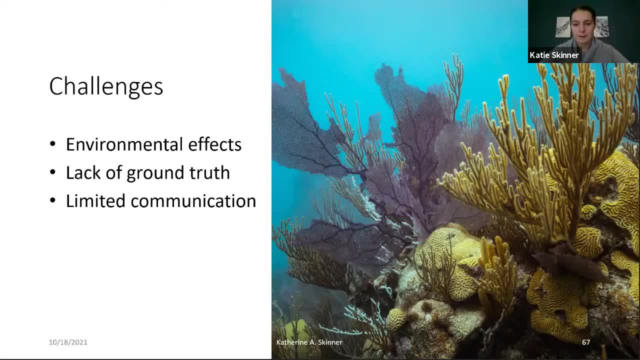 And they vary across different sites. So we need to be able to develop methods that not only can operate in a single site, but can generalize across different sites as well. So this is really a unique challenge for underwater vehicles. The second challenge is that we have a lack of ground truth data. 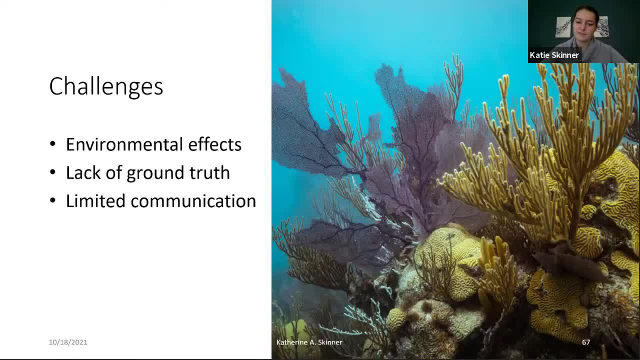 whether that's because we have different sensing models, we have different sensing modalities that we work with underwater since, such as science and sonar, or because there's just the lack of lack of resources for generating large labeled data sets of marine environments. 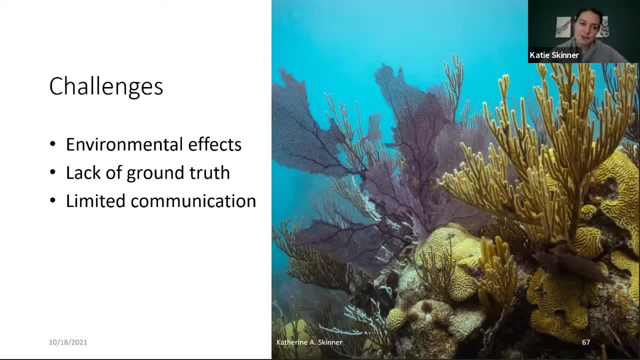 Kind of in contrast to what we've seen in the autonomous driving community. where we were, the access to large labeled benchmark data sets has really spurred a lot of recent advances in computer vision for autonomous driving. We would like to see those same successes underwater. 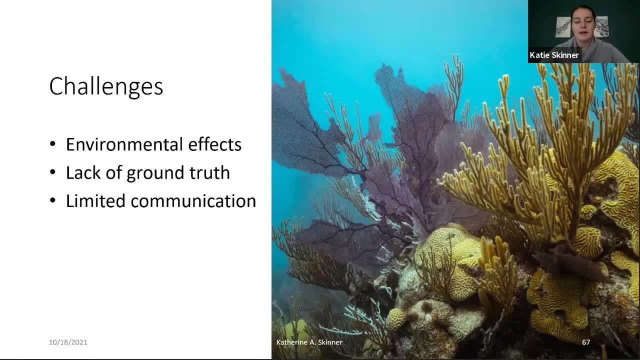 But one of the challenges we might have to overcome is this lack of ground truth And, lastly, what I didn't quite touch on, but that's really important to keep as a reminder in the context of working with marine robot robotic vehicles, is that we have limited communication to our vehicles when they are conducting their underwater surveys. 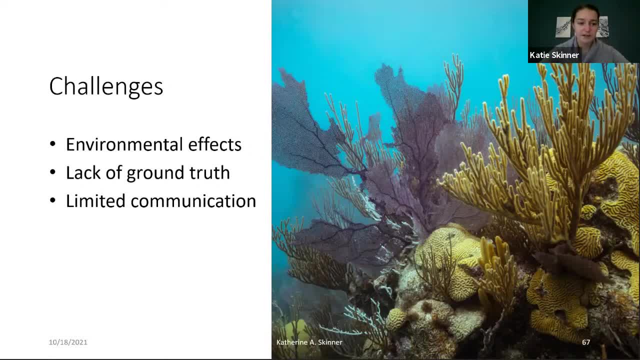 And this just really motivates, motivates the need for enabling these vehicles to have more autonomous capabilities so that they can perform large scale, efficient, repeatable surveys on their own and explore reason about what sites are interesting, to go explore those sites further without human input. 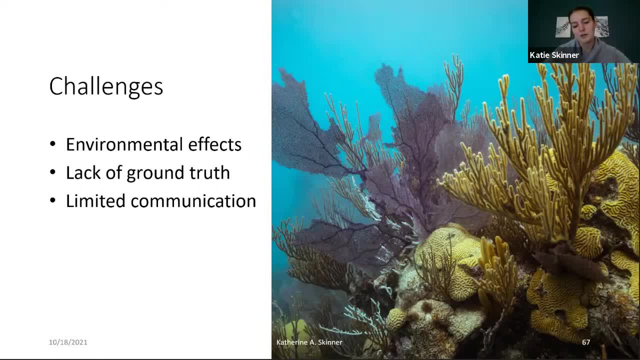 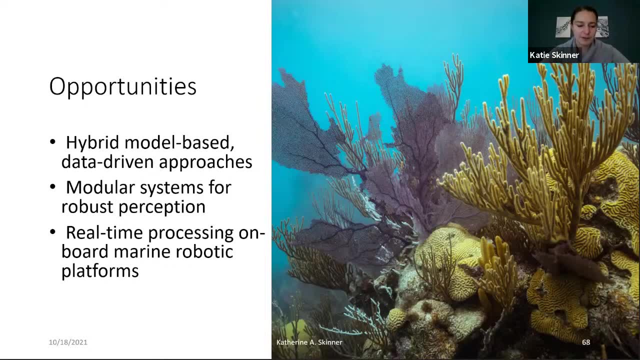 So this limited the limits to communication underwater are really a challenge. But all of these challenges, I think, can be turned into opportunities for developing state of the art, state of the art methods for marine robots. And the first opportunity is really to think about how do you incorporate model based approaches with data driven solutions to enable unsupervised or self supervised methods for marine robot perception. 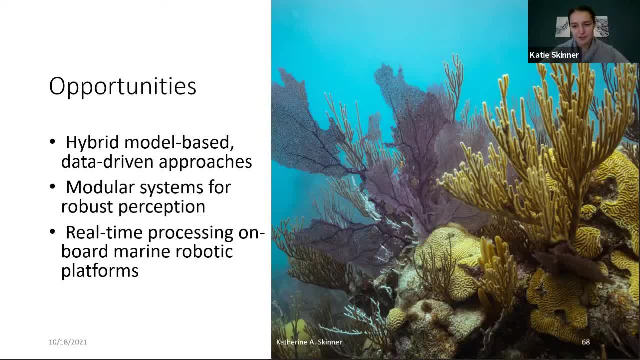 The second is, I think, promise of modular systems for robust perception. So I focused in my work, such as underwater stereo net, to make these systems as modular as possible So that perhaps we could swap out. swap out systems such as the front end systems for underwater slam with deep learning modules. 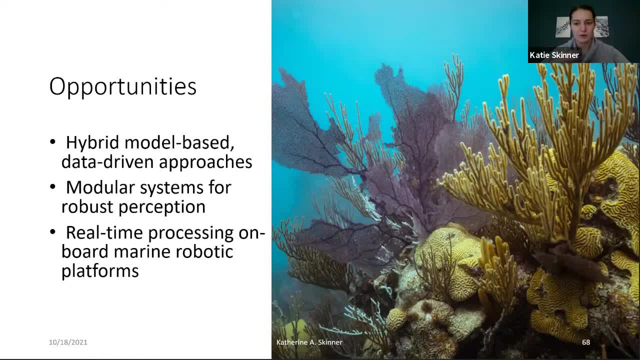 instead to work towards more of a modular solution, while still leveraging the frameworks that we've developed over the years in robotics that really do have great success as well. And lastly, as I hinted with the limited communication, we have an opportunity here to 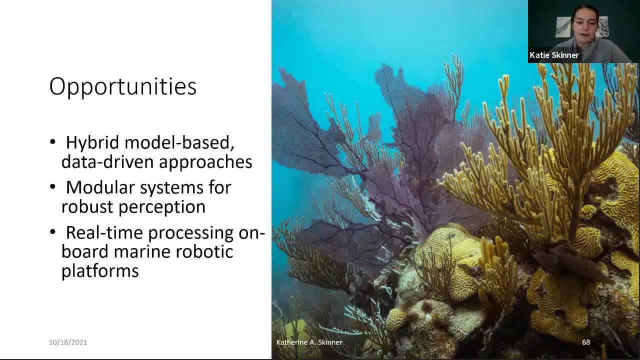 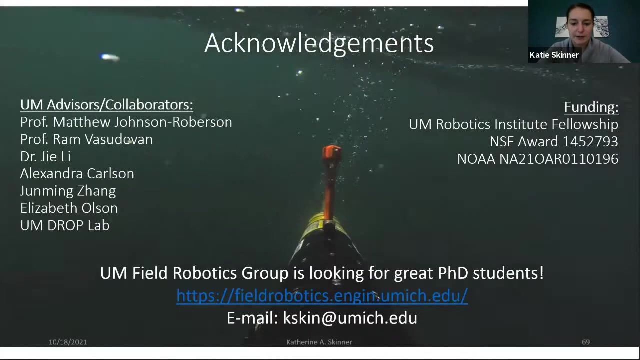 we have an opportunity here to develop methods for real time processing of onboard- onboard marine robotic platform. So leveraging these new technologies to enable our equip our vehicles with more real time autonomous capability, I think is a really exciting opportunity. So I just want to acknowledge my UM collaborators, as much of this work was done during my PhD at U of M. 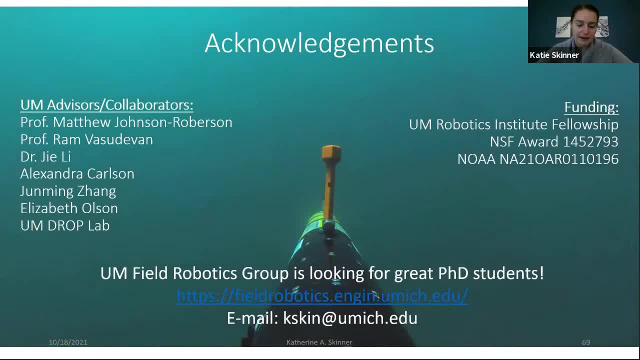 And then my previous and current funding as well, And just a plug that the UM field robotics group is looking for students this year, So always excited to hear from potential future students. Thanks, Catherine, for the wonderful talk. Those are really exciting results there. 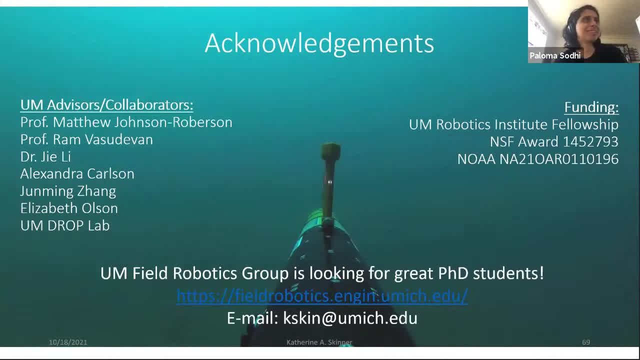 So we have a couple of questions. Maybe, okay, maybe I'll start with a. a simple question on like so is a: is a projective camera model still valid for underwater applications? So the pinhole camera model isn't exactly accurate. 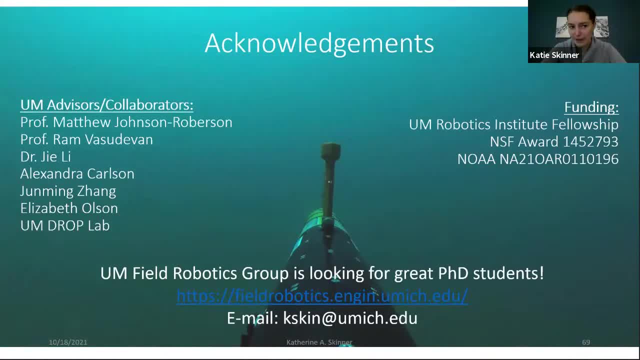 but it does work well in practice. One of the other challenges I didn't mention here is refraction, And that can break down assumptions for the pinhole camera model. So refraction occurs because we have to put our camera then underwater housing. 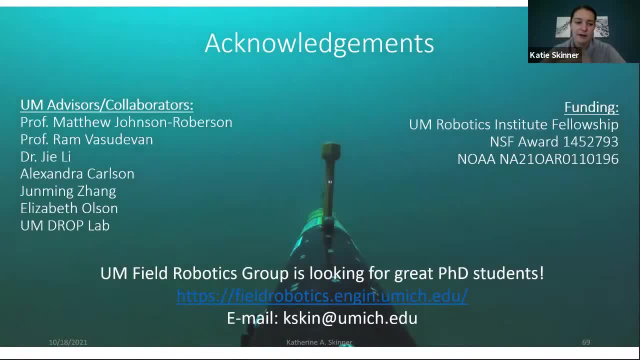 the light rays go through an air glass interface and then a glass- water interface. So there are some ways to overcome these challenges. One is we calibrate our cameras underwater So this can kind of mitigate some of the error from refraction effects. But definitely there's a lot of. 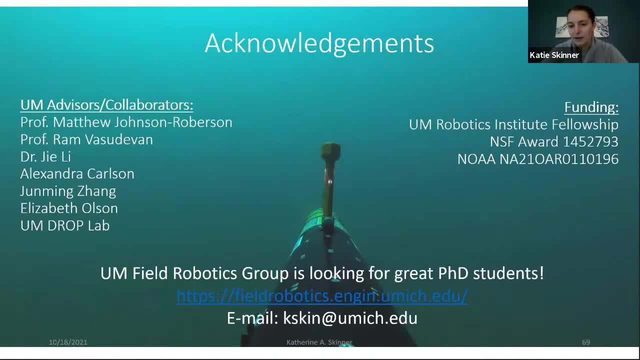 a lot of work in how to accurately model, accurately model these effects for camera calibration And for and for generally mitigating errors that arise from from refraction and underwater effects. So you so you need that calibration step within the underwater. 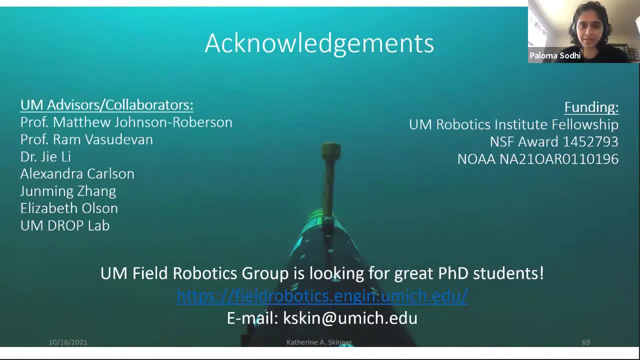 with the underwater images themselves. Yeah, we, we actually waterproof our calibration boards and perform the calibration underwater. There's also dome ports are widely used Underwater as well, So that can also help to reduce effects of refraction too Cool. 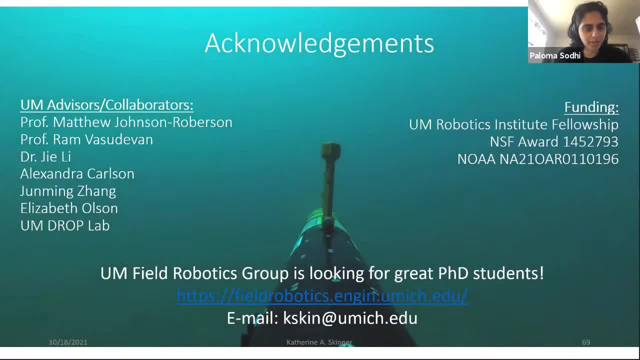 Thank you, And then maybe a follow-up question on so the, is this more on your water GAN work? So the magnitude of backscatter and attenuation may vary depending on how turbid the water is. So does water GAN give similar results for different turbidities? 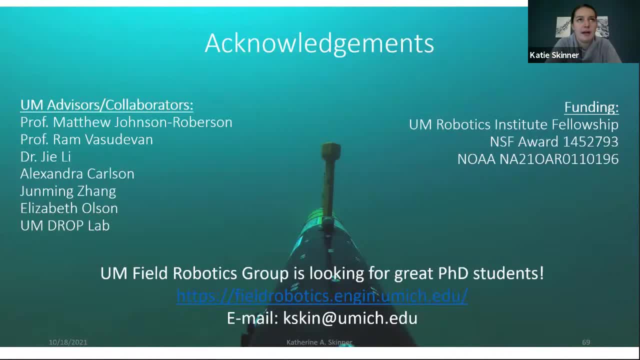 So we tested water GAN in kind of a tank environment And then in real environments from data collected in Jamaica that did have pretty high turbidity And we saw. what we saw was that the results were consistent across different sites. So one thing to note is that we did retrain. 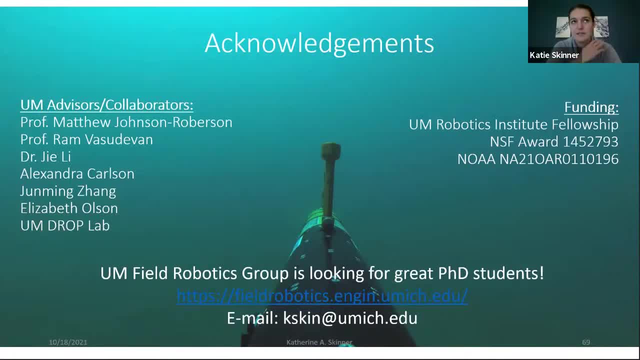 we retrain it per site. So we assume that we have similar water column effects in a small local area, And then we retrain that, And then we retrain the network per site. So that is, you know, one way to help us overcome. 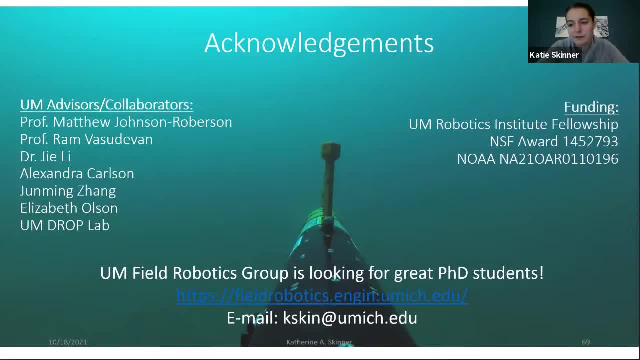 Overcome challenges with having different haze effects across different environments, But we certainly like to work towards developing generalizable methods that could be thrown into any underwater environment Interesting. I'm curious like how. how often do his effects vary significantly between the environments? 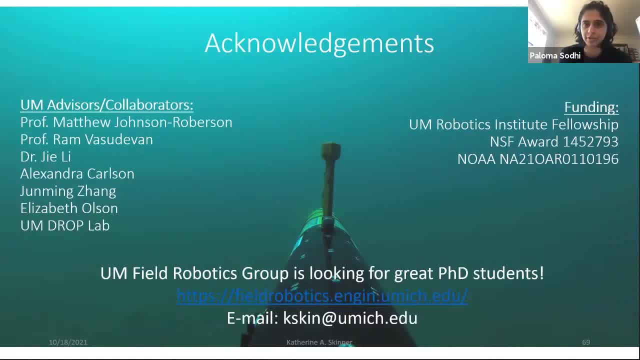 that you're doing it, So you're testing in the same area. You're not changing your job Location. Yeah, they can still vary, even for one environment day to day, If you have, you know, depending on weather patterns Or even. 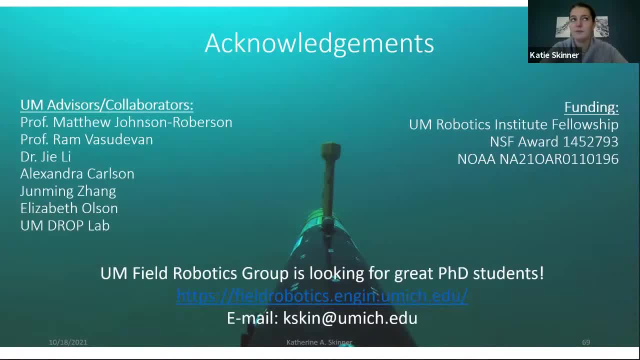 you know, if you have strong voting traffic, you could say. So. it really, it really just depends on the environment that you're in And what. what else is in that environment? Oh, thanks, Okay, Then you have another question on. 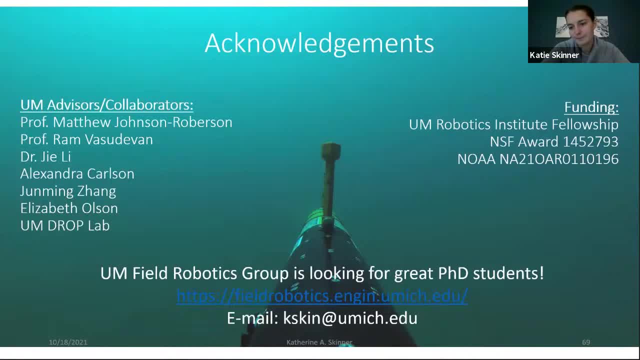 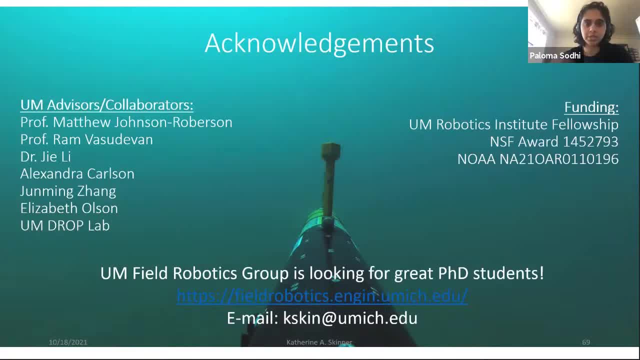 Yeah, So is there actually any like any kind of connection between the image restoration model and the stereo vision model? And how does the stereo model learn to restore color under an unsupervised setting? Yeah, So the main, the main way we leveraged kind of the physics based model there was. 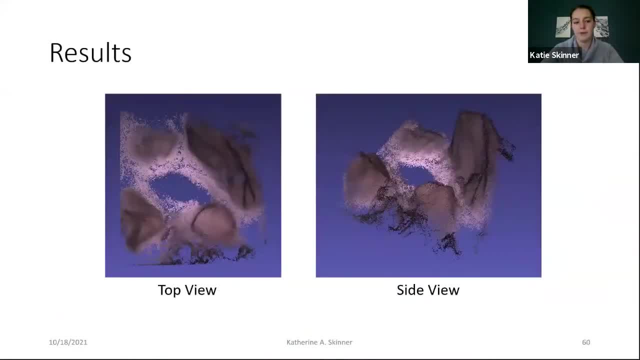 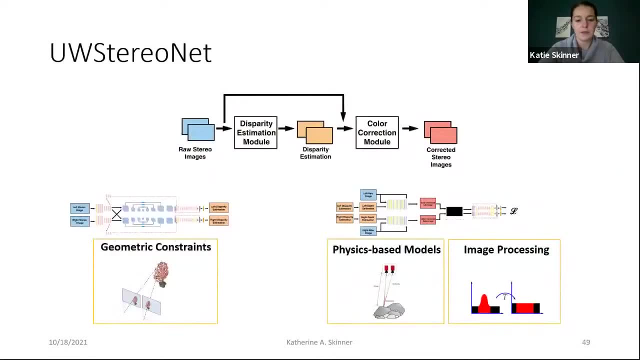 just the Notion that the image restoration process is range dependent, So that network is more of a traditional. But we take as input both the disparity map and the RGB image because we know that the restored image should have some notion of what that depth map is. 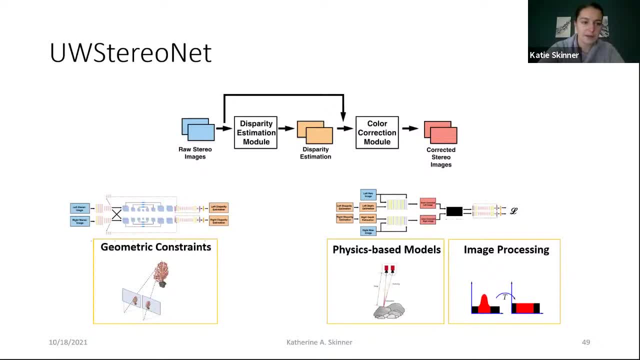 So, yeah, this work was a little bit more abstracted, I guess, from the physics-based model, but more looking at what is important for modeling, or learning to model these effects, And that's really the range and the depth dependency is really important for getting consistent color correction from underwater scenes. 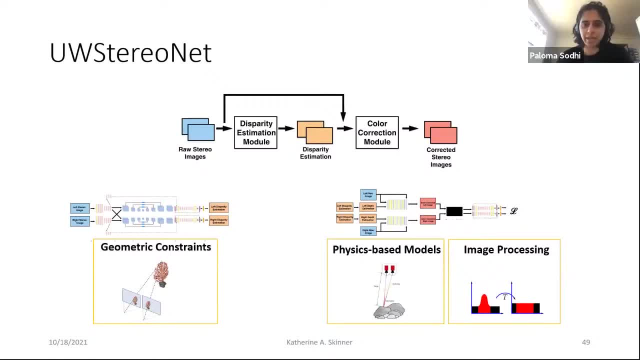 Interesting. So, like the depth, information is probably encoded in the color artifacts that you see, naturally. Yes, Yeah, that's what we hope For this work too. we also looked at incorporating image processing methods, So we have one component of the loss function. 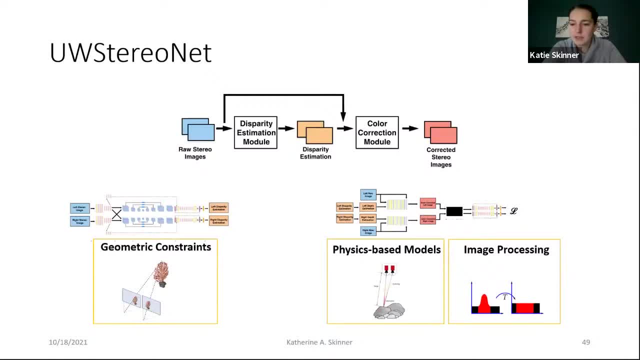 The other component of the loss function is working towards the gray world assumption, So that also helps to constrain the image restoration component. So it is, it's taking some inspiration from the gray world assumption, from image processing, but also ensuring that it does this in a consistent way, according to taking the range of input. 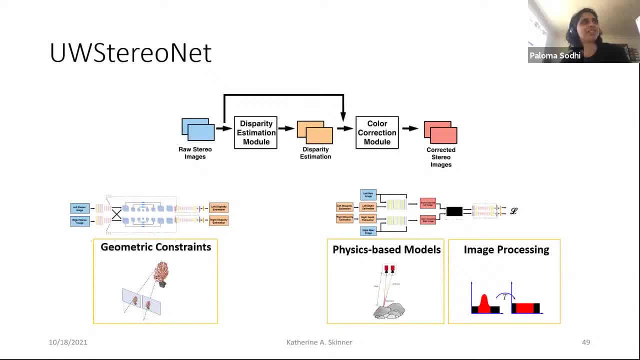 Thanks. We also have a couple of interesting high level questions, So one of them is like: so is there any insight from the underwater applications that you've worked on that can be transferred to other domains, such as dealing with obstructions and visual slam or or some other effects like that? 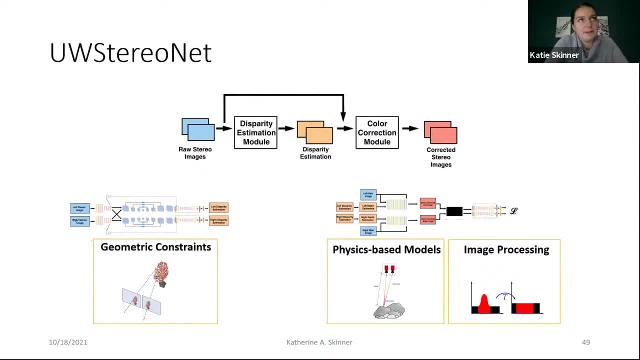 Yeah, I mean I think there's a couple of some more. more of the direct parallels are really fog in air or haze in air follows a similar model to underwater underwater effects. So that's maybe one of the more More direct parallels, But certainly carrying forward the idea of 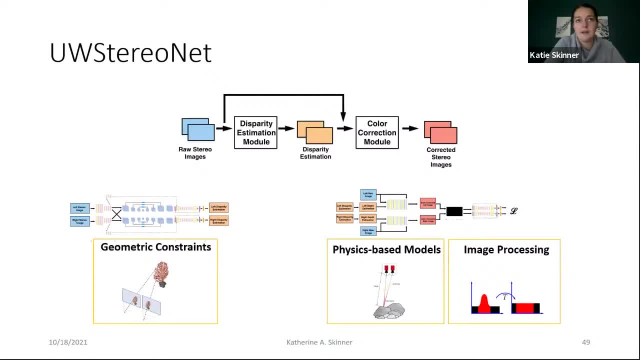 you know, generating synthetic data for training, deep learning networks, I think can definitely be transferred on land, depending on course, depending on what environments you're looking in. So I've had prior work looking at how we can learn to model sensor effects. So modeling noise and individual cameras are modeling. 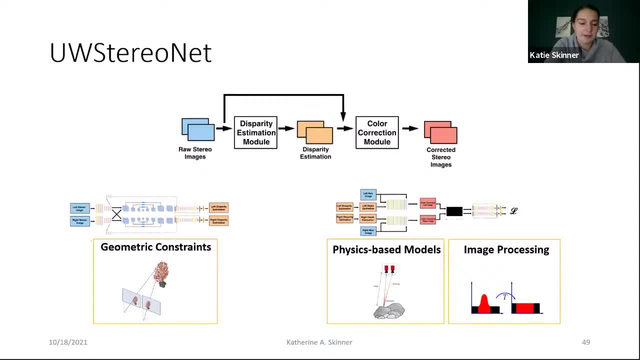 Color tone or blur and chromatic aberration, How we can learn to augment simulated data with these sensor effects to improve object detection from autonomous drive for autonomous driving applications. So I think just learning network or using networks to learn to generate realistic effects can definitely be transferred to different domains as well. 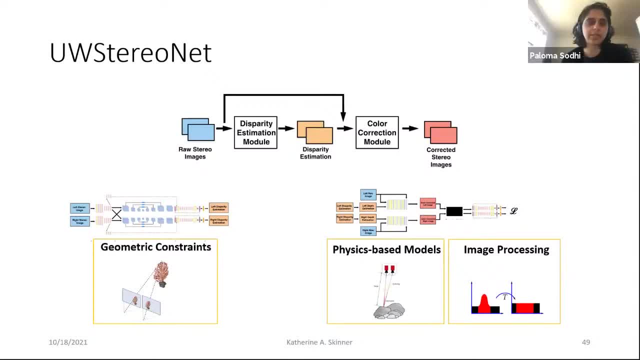 Interesting And maybe one follow up on that. Do you see, like physics based, like scattering models and things play a similar role for those applications as well, like fog and haze outside of underwater environments? Yeah, I think a lot of the recent work seizing deep learning for de-hazing even on land really do look towards inspiration from the physics based model of image formation on land in the presence of fog. 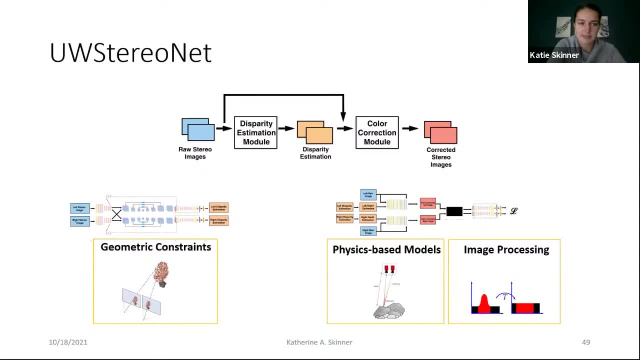 So that's exciting to see. I think that this idea of incorporating This idea of incorporating physics based models is a really, really useful idea and can really help to structure deep learning frameworks, to improve the training and kind of point you know, point towards what we actually want the network to learn. 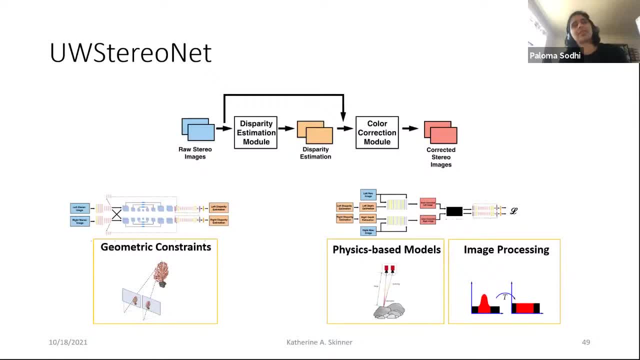 Oh, thank you. We have another interesting question on like: so for the level of detail that you're looking to achieve, and reconstruction. So, for the level of detail that you're looking to achieve and reconstruction, Is there any inspiration in animals? Is there any inspiration in animals? 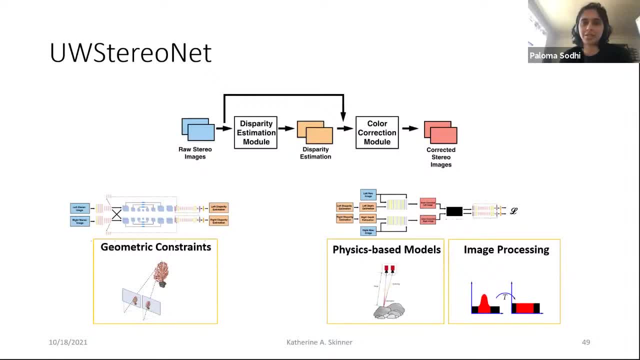 So any specialized sensor found in nature for that detail of reconstruction? That's a really good question that I don't know the answer to, But if anyone knows, I would love to love to hear about bio kind of bio inspired vision ideas as well. Yeah, and this one question more on the platform. 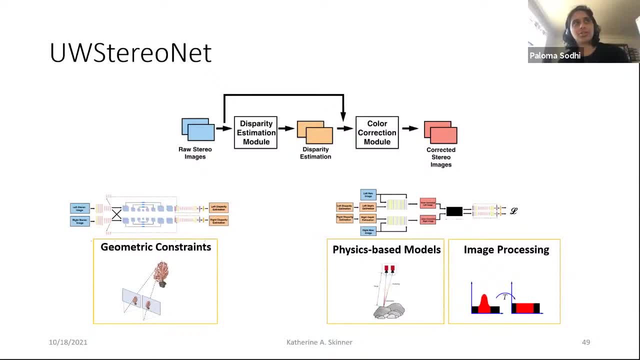 platform. So what kind of computing platforms do marine vehicles usually carry, and are the vehicles energy constrained? So it depends on the vehicle, because there's kind of a wide range of tasks we want to achieve. So there are remotely operated vehicles that are tethered and those 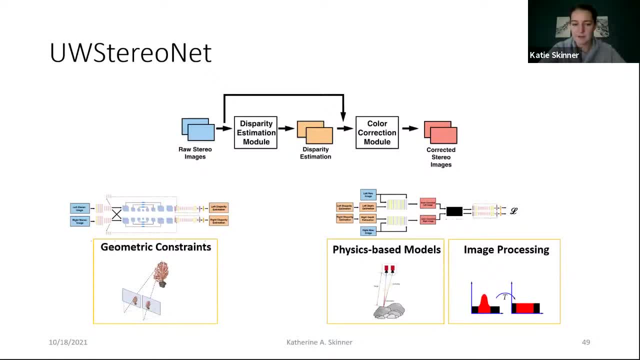 vehicles are typically larger platforms So you could have greater computing resources on board. But for kind of the lightweight autonomous underwater vehicles and micro AVs you're definitely constrained by size, which of course can have, you know, working towards a smaller size. 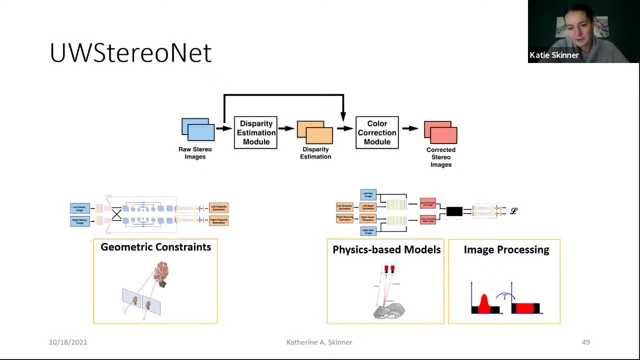 can greatly reduce the cost of these vehicles, But it can also enable them to go to a different, a wider range of environments in general. So definitely limited in computing resources on board. For the methods I've presented here, we mainly tested the computing resources on board. We tested the computing resources on board. 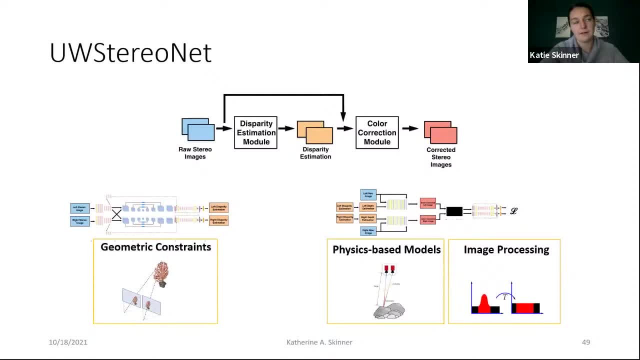 and we tested them offline or off, not on board the vehicles themselves. So that's kind of. the next step is to maybe put a Jetson on board our blue ROV and enable on board processing for some of these methods. That's really exciting, I think. yeah, Josh has been building such vehicles too in. 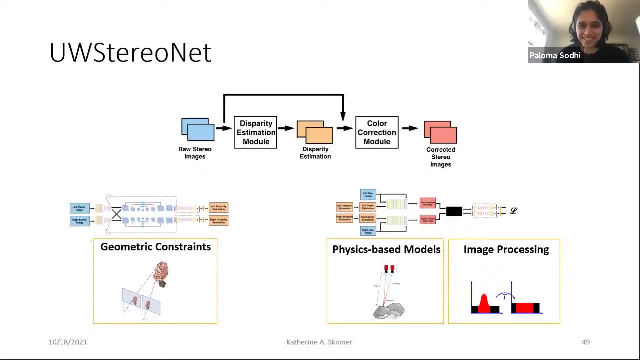 his lab, So I don't know if he had some thoughts to add to this. Sure, Yeah, Yeah. So I think one thing is the size of the vehicle. So I think it's really exciting. I think it's really exciting. 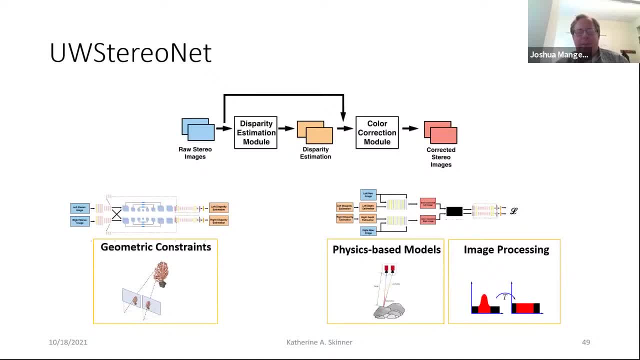 So the size of the vehicle really does limit about how much you can carry. And for one of the things, we have been trying to integrate a Jetson Xavier into a blue ROV system so that we can try and add more processing on board the actual vehicle itself. But that's. 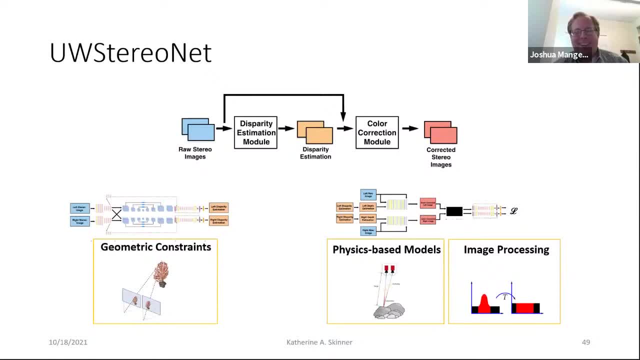 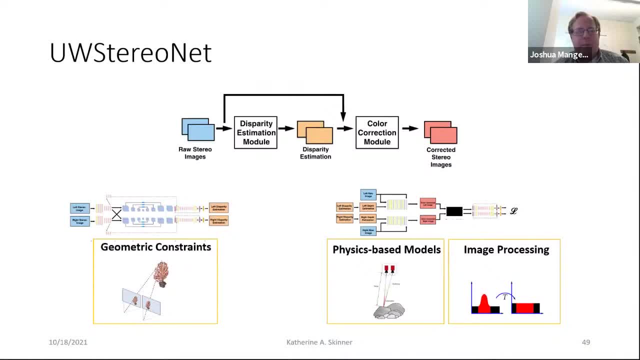 able to. if you want to be able to do processing at the surface, then you need to have more costly tether systems as well, which is another thing that eventually causes problems over time. So, one of the things you can, you can go to optical fiber based tethers, for example. 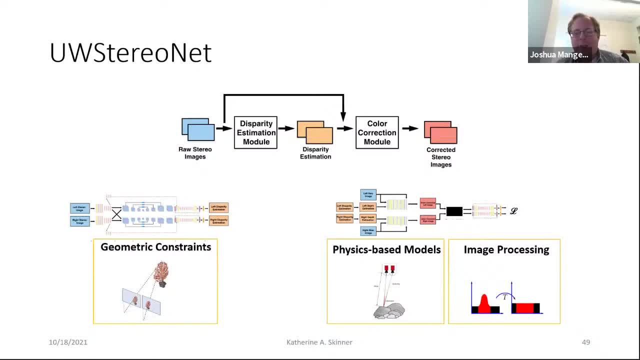 but those can be easily damaged and things like that. So so it really, and they limit how far the vehicle can really travel. So if you want to be able to have it autonomously nap a lot of large area, then having a tether based system often is not necessarily what you want to be able. 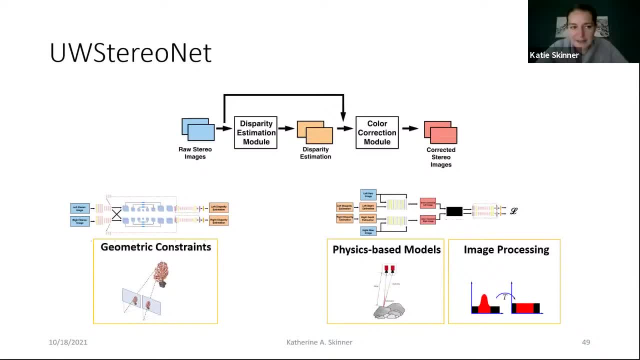 to do So. there's definitely trade-offs between those two And there's definitely becomes a problem, a problem as well on its own. Yes, absolutely So cool, Thanks, Yeah, I think it's kind of exciting seeing the development of these underwater ROVs, like with more accessible. 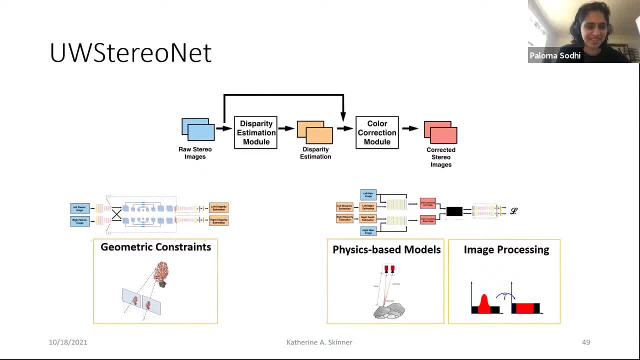 platforms and open source codes. Okay, Catherine, maybe I'll switch back to a bit more technical question on your work. So there's one question on. so, concerning depth generation, was the left-right consistency idea similar to what other self-supervised depth generation networks that target other applications like 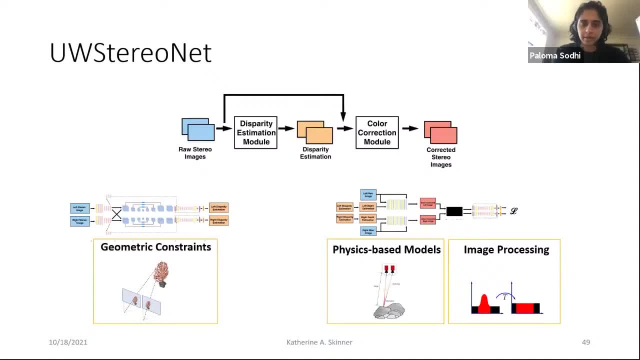 self-driving cars use. Yes, Yeah, So this was. yeah, it's very similar, So it's a differentiable bilinear sampling for developing a loss function for left-right consistency So you can use the estimated depth maps to warp- essentially warp. 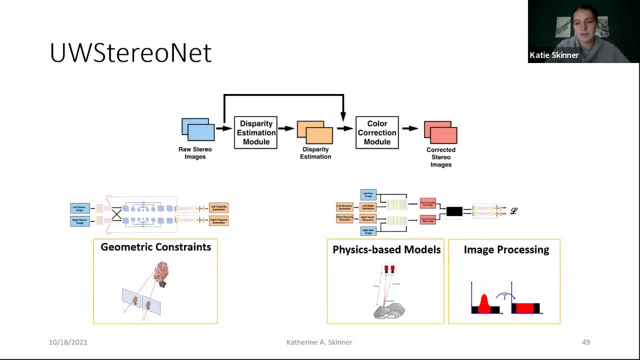 each of the images to the corresponding views, And then that can be kind of a self-supervised signal for learning accurate depth maps, because if your depth maps are accurate you should be able to warp the images: the left image to the right image and the right image to the left image. 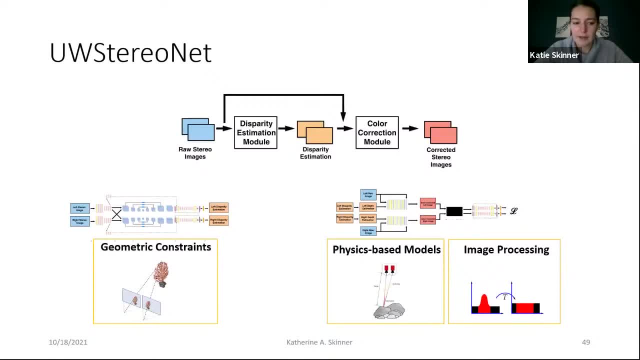 and have accurate reconstruction results for the warped images. So, yeah, that's something that's been done And I think it's really important to have that in mind as well- used for terrestrial applications as well. One thing that was really interesting to us was that 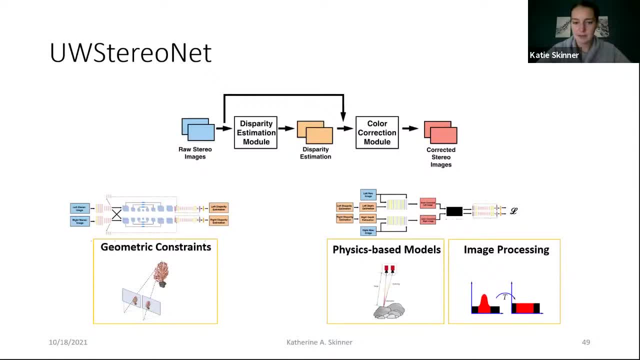 we actually pre-trained this network on cityscapes data, which you would think would be very different from our underwater data in many different ways. The baseline is very different And, of course, the underwater effects are different, But we actually had pretty good results just with. 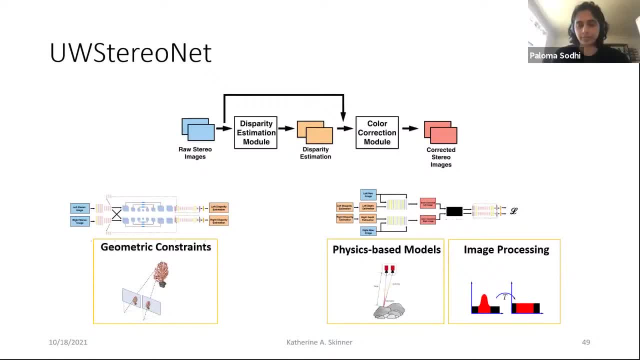 pre-training on cityscapes data. So I think these types of self-supervised networks are really really useful in terms of generalizability, even across different configurations. So that was exciting to see. We did have some improvement, of course, once we fine-tuned on our own underwater. 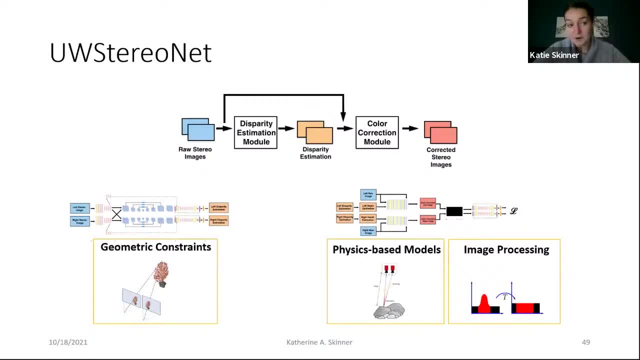 data, But it was exciting to see just how well it worked, even with pre-training, because I didn't expect that at all. Interesting. Yeah, I think maybe this is an example of insights transferring across applications as well. Yeah, Okay, So another question that we have is: so is there any other information that you 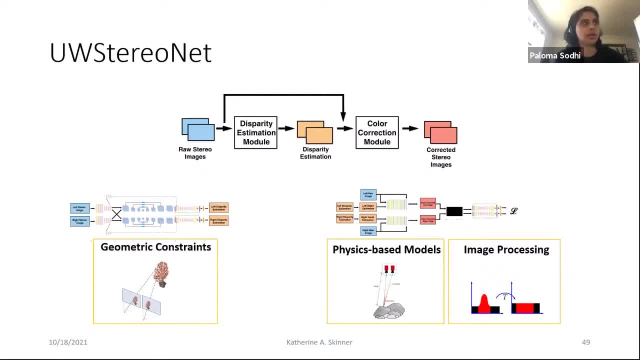 combine with array sonar when you're trying to recognize shipwrecks. So how do you get ground truth for those shipwrecks? Or was that using any ground truth? the results that you were showing? So we don't have. this is kind of a new project: we've started, So we haven't done. 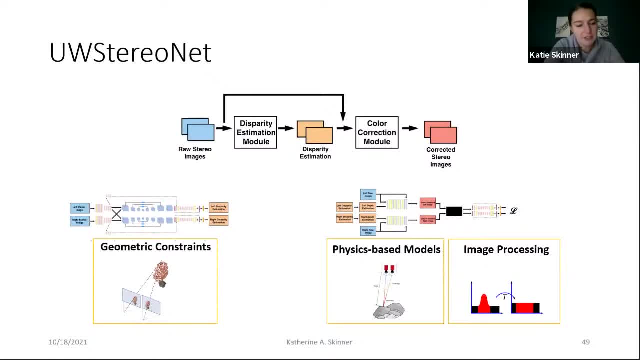 so we're developing methods now to do deep learning-based shipwreck detection The method. there have been a couple of methods that have come out that really look at the shadow effects from objects in sonar imagery. So that's kind of one cue that we have looking at sonar imagery for. 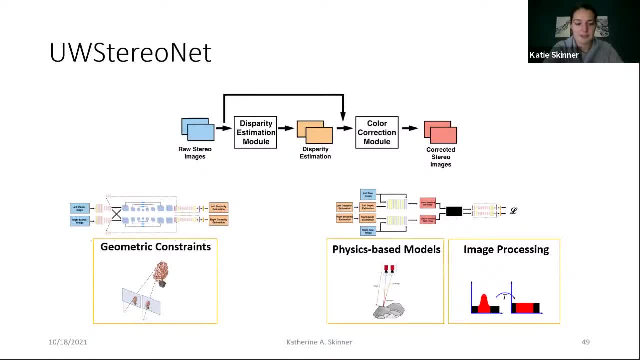 detecting interesting objects. But there's of course a lot of distractors and a lot of challenges, especially with complex terrain for interpreting sonar imagery. So one kind of challenge we've seen too is that in having experts label sonar imagery it's challenging even to know where to define the boundaries of objects. 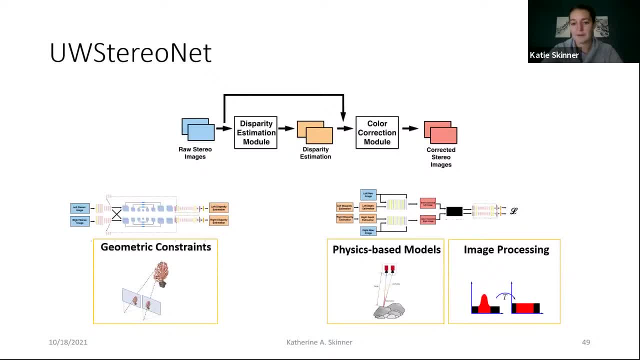 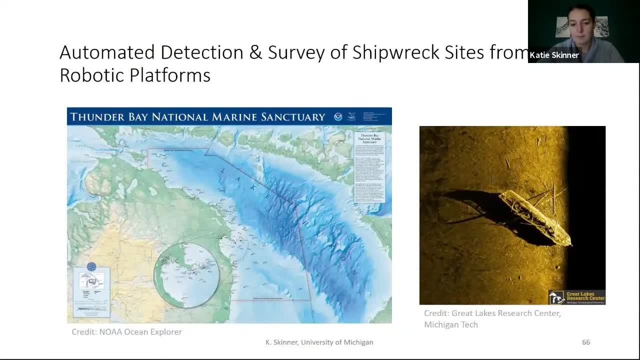 sometimes for expert viewers because of the shadowing effects. So even the process of having a human hand label, a large sonar dataset, would be pretty challenging. So this image was from our collaborators at Michigan Tech in the Great Lakes Research Center And this was really a close range, high resolution survey of a shipwreck with a known location. So 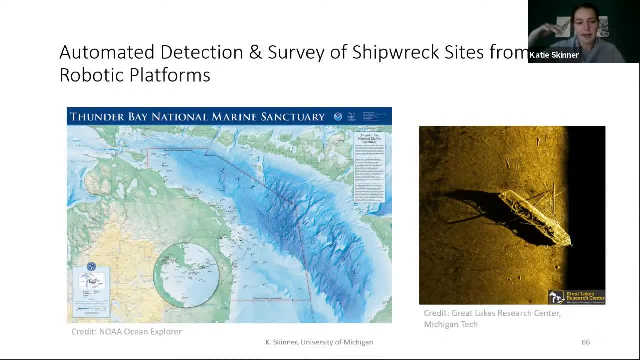 the idea for us would be to be able to take higher altitude surveys so we would have low resolution imagery coming in and we want to be able to detect shipwrecks from that low resolution sonar imagery. But a lot of really interesting challenges there to think about what cues we have. 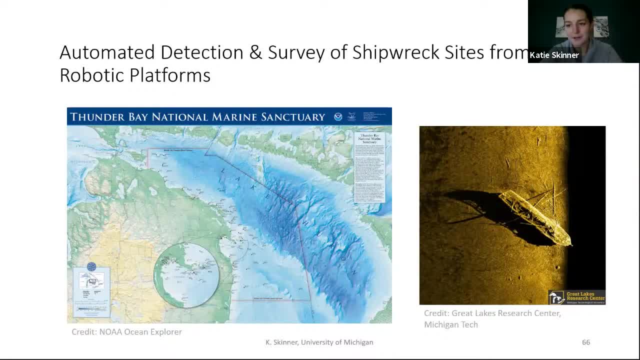 from sonar imagery that might be different than what we have from RGB imagery, Yeah, and I think that's a really interesting problem too as well. So in the underwater domain, like Katie mentioned there's, it's really difficult to. 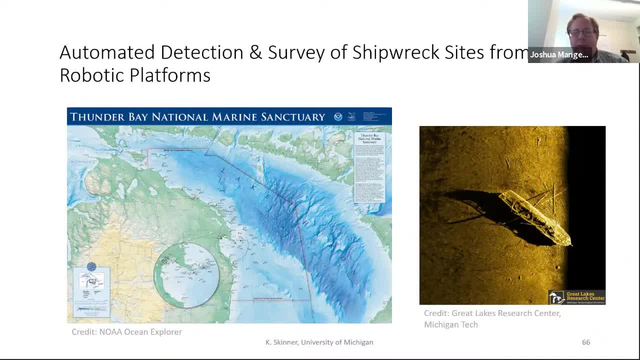 get labeled data, and even large amounts of data is difficult to get in general. So, Katie, one thing I wanted to ask was just: do you have any ideas about other than automatically generating that data? do you have any ideas about sim to real transfer of data or anything like that? 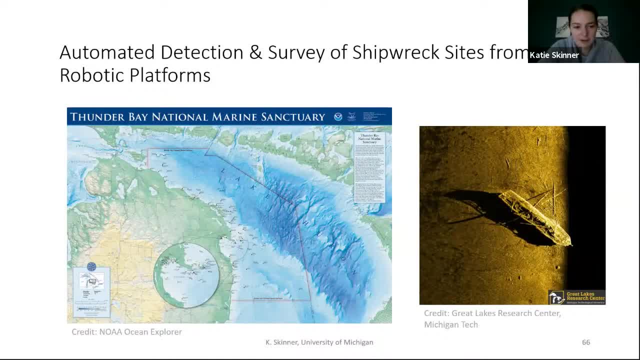 Exactly So where that's kind of, one of our focuses for this project is leveraging simulated data. There aren't a lot of open source sonar simulations platforms either, So we're actually releasing an open source sonar simulator right now, So 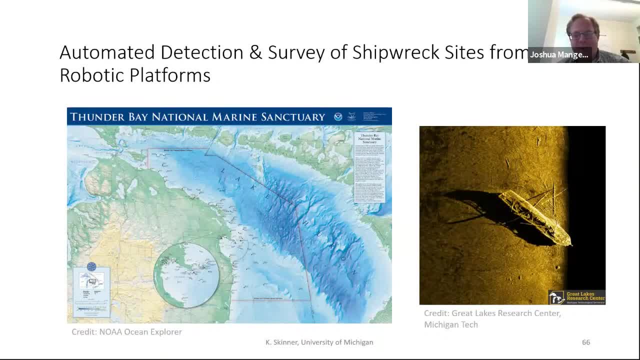 if that's something you're interested in, I can get you access to that as well. Yeah, that's definitely something I'm interested in. Yeah, and one thing we're really interested in too is- and we've seen kind of this trend for terrestrial applications too, for autonomous. 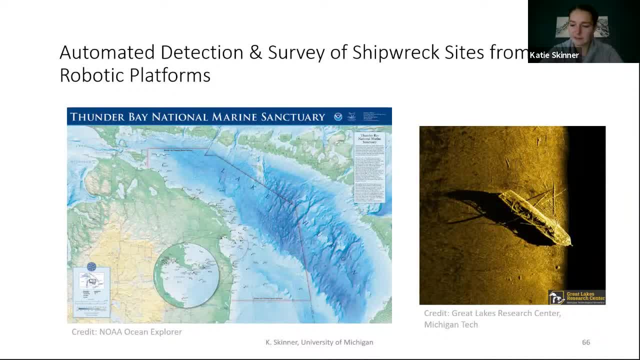 driving is being able to leverage low fidelity simulation, So it's going to be challenging to make a perfect simulator for any environment or any task. So how can we, how can we ensure that we can still make use of lower, like low fidelity simulations without having, you know, a perfect? 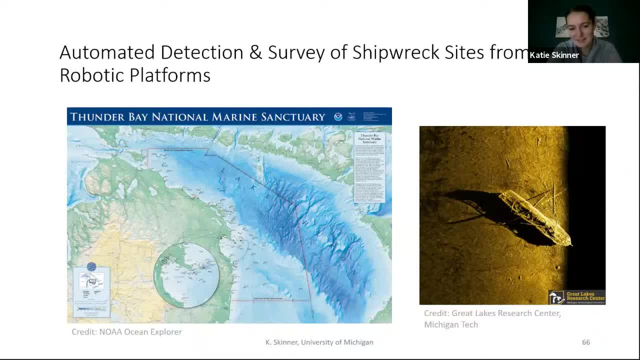 replica of our underwater scene. But yeah, Josh, that would be very helpful. Yeah, yeah, I'd be happy to send it to you. It's called, it's called Hollow Ocean, and we've been, yeah, we've been. 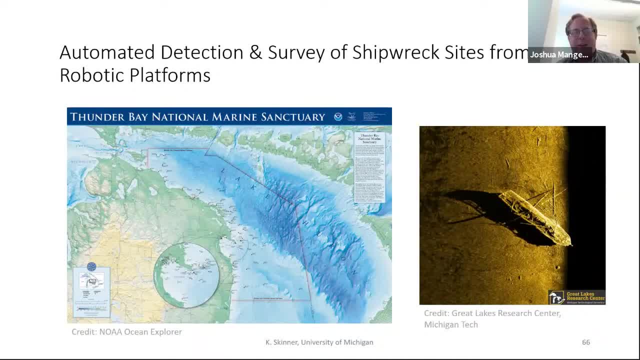 right now we have imaging sonar and we're hoping within the next month or so to have side scan as well. So yeah, I definitely hope that the that the sim to real, sim to real can transfer to the underwater environment and underwater perception specifically. 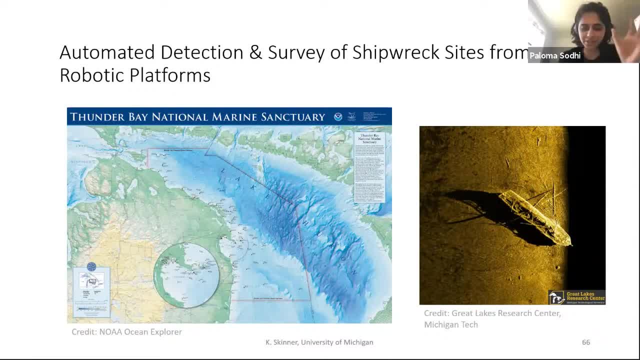 I, you know, I feel like the thing that you were showing, the results that you were showing with the water gun, like with the air images and underwater images, like there's, there's kind of a gap there also. So there was already like some gap that the network was sort of interpolating. 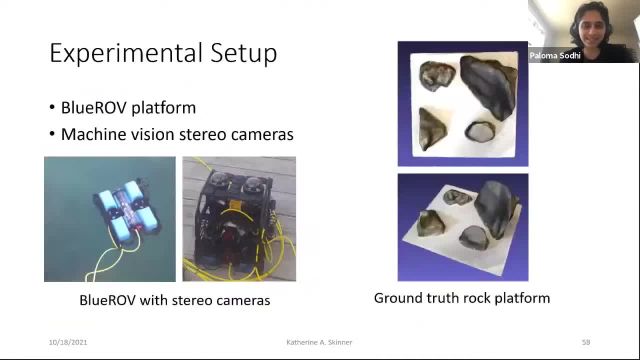 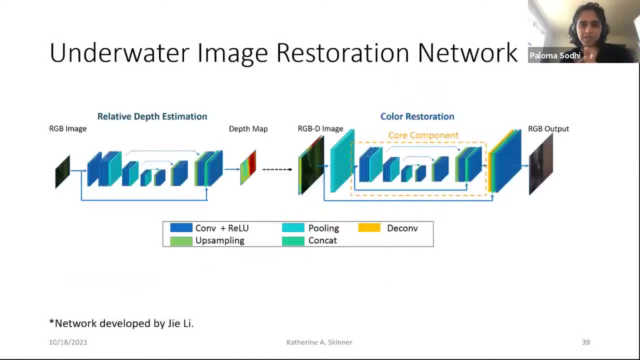 between the images, I mean- and this is a different use case- but like it's interesting, like if there's this simulator and maybe that's the gap that it's going to cover, like going from a simulator to actual images, rather than air images to water images, 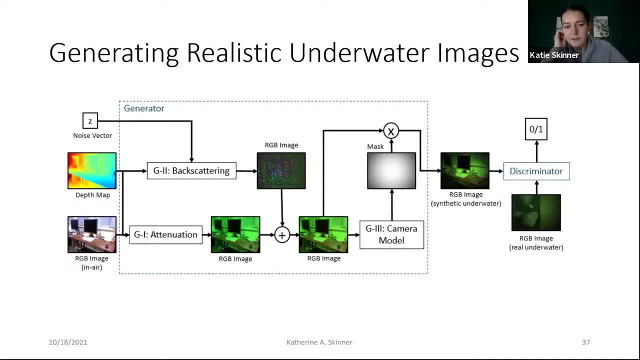 And that's yeah. yeah, this was and this was one reason we really looked towards structuring. So the generator is pretty highly structured, right, There are pretty- there are not that many parameters that it's learning compared to a traditional convolutional network, because we 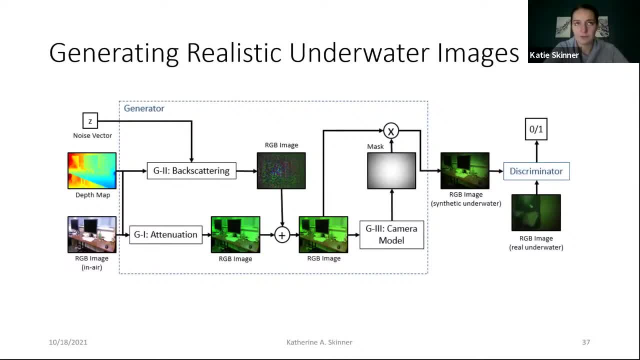 integrated the physics-based model here, And one of the reasons we did that was because we saw that the like- looking at typical like cycle dam networks, for example, going from air to underwater- what we saw was that the in-air imagery has such a different. 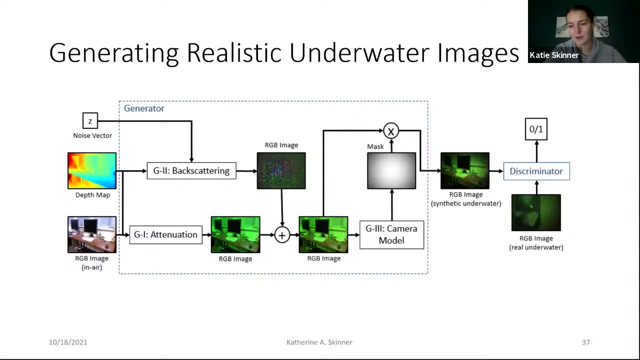 spatial distribution of features than underwater imagery, that the network was also kind of learning to transfer the structure as well. So, yeah, this that was kind of one reason we looked to structuring the generator. So it has kind of a limited. it has limited ways it can. 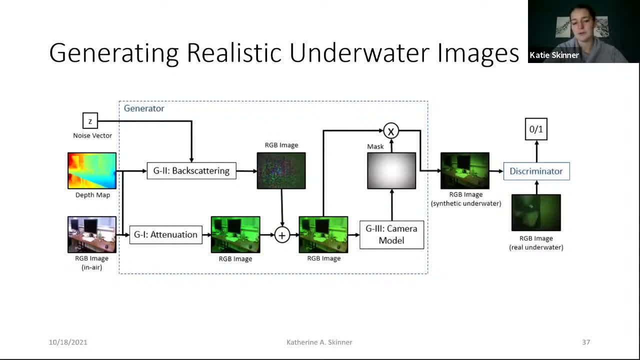 change the image. So it's really only allowed to change or to add attenuation according to the physics-based model, based on the learned attenuation parameters. So that was kind of. one nice benefit of incorporating the physics-based model was that we could constrain the network to only change specific aspects, which here were the underwater effects, not the spatial arrangement. 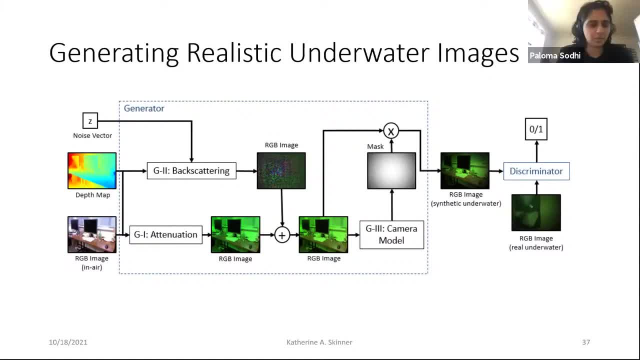 Yep, Makes sense. Yeah, Cool, Josh, just to ask, like, is there a simulator, physics-based or the? Yeah, Yeah, So it's. yeah, So it's based on Unreal Engine. So, so we have, you can generate automatic or you can, you can generate actual 3D structures. 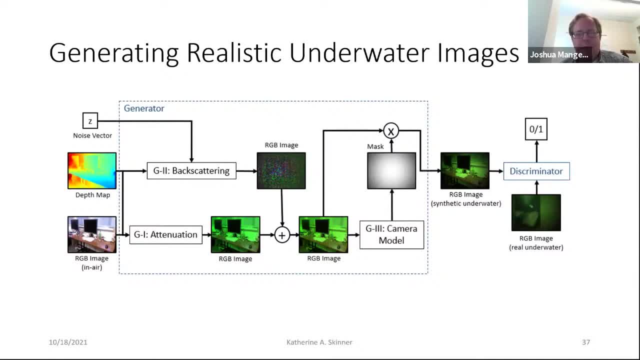 within the space, And then we're using the projective model of a sonar in order to try and generate what that data looks like. So one of the things we want to be able to do relatively soon here is incorporate noise in a more accurate way And cause that's. 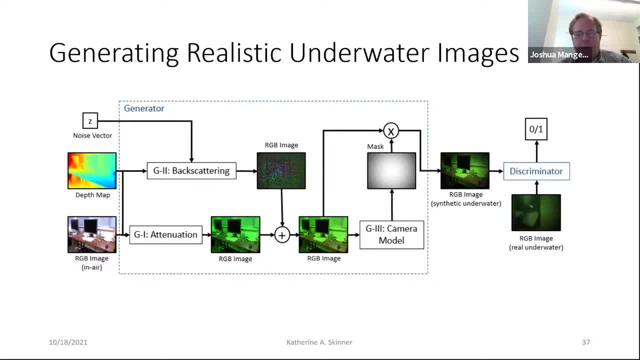 that's a more complicated thing for sonar, especially with reflections and reverberations, lots of other things that can can add noise to, to the to the sonar. But right now, right now we're able to generate, based on the projection model of a sonar, we're able to automatically 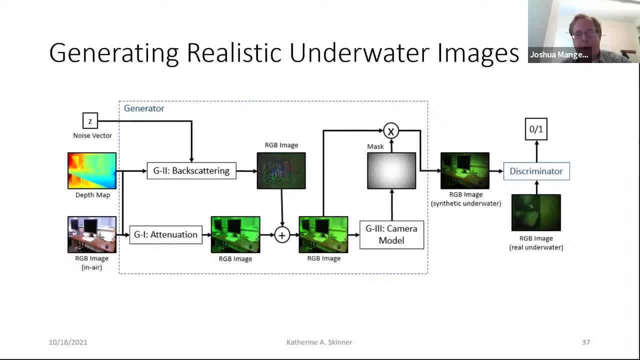 generate imaging, sonar multi-beam imagery of of 3D structures and then output that as as an image. Cool Sounds, cool, Okay, And maybe yeah, switching gears a bit, Katie. we have a question still coming in, So I think this one for this question. 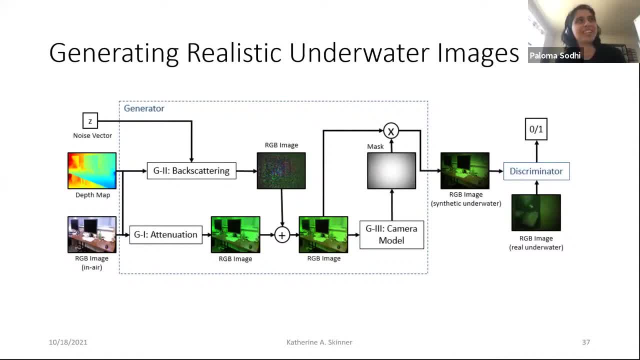 maybe your field work comes in handy. So much of the the question is, much of the interesting biology happens at the interaction between mediums, So coastlines, shallow waters, kelp forests, et cetera. Any particular challenges that you see for enabling robotics in those areas? 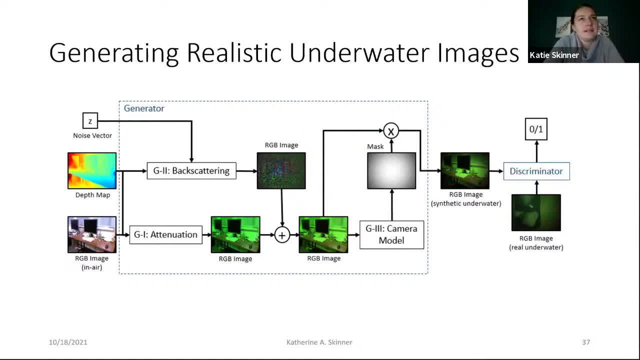 I think there's kind of recent interest in platforms that can go from underwater to shore environments. I think they're called amphibious platforms. So that would be really interesting to see how, you know, we could design perception systems for those types of vehicles. 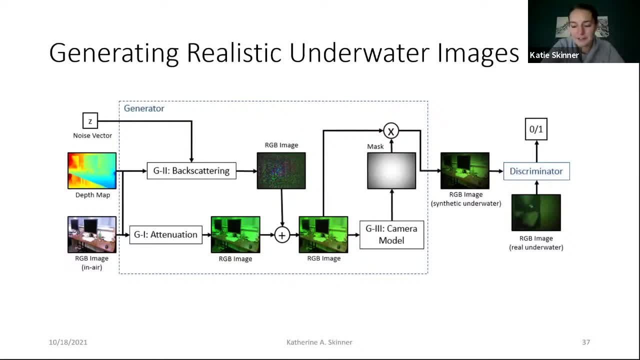 that would be going in and out of the water. I think that would be one really interesting kind of interesting thing to see come out of those applications. Some of the challenges there are just, I guess, general challenges in working in near shore environments And that really, just you know, might change the type of platform that. 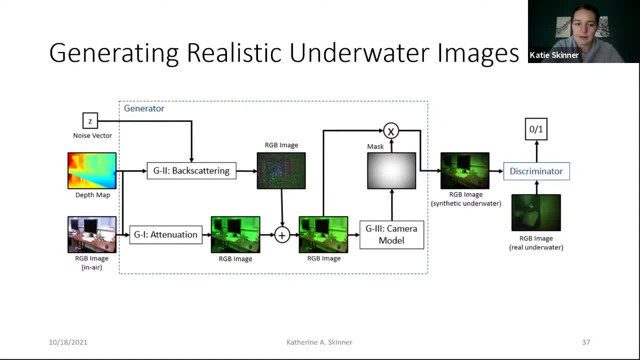 you choose to use, depending on especially how. how much vegetation is there. This could be a challenge for autonomous vehicles going into some of these environments. Yeah, I was going to say the same thing. I think I think the the true. these vehicles tend to be somewhat expensive and it's somewhat dangerous. 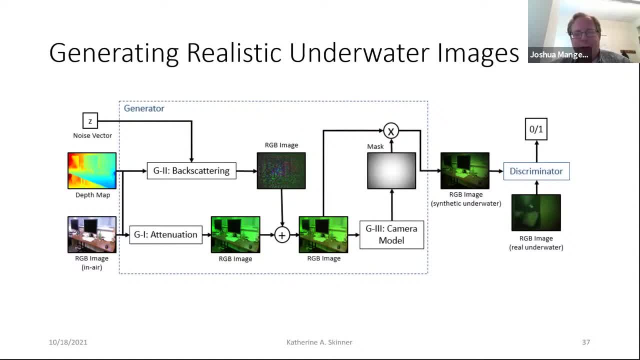 you know, to operate them in in those environments, And especially with vegetation or shallow water. those are places where it's easy for the vehicles to get damaged right, Or for for waves to smash them into the, into the shore, or or for them to their them to get. 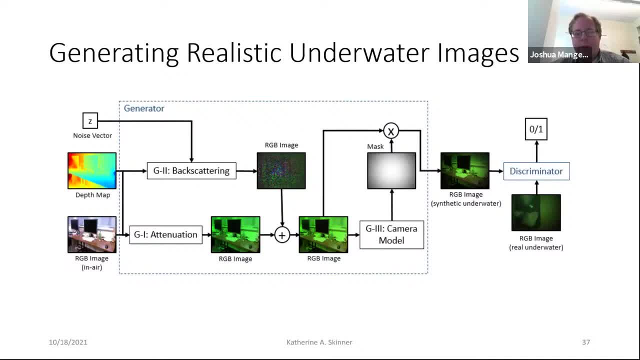 tangled in some way. So that's that's another situation. that's a problem for general autonomous underwater vehicles, but especially when you have tethers, that that becomes a big problem to be able to operate in those locations. So so designing specific vehicles in order to operate in those spaces is a really 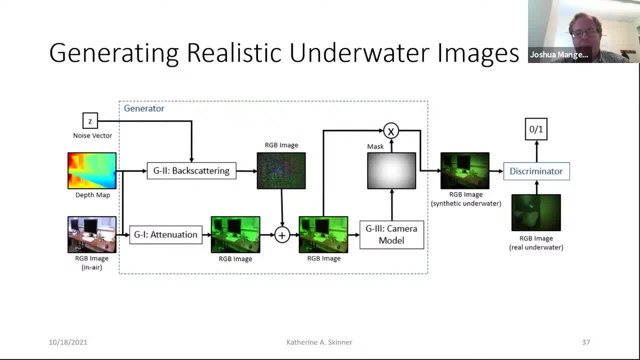 interesting idea And then there's interesting perception problems within that space too. Yeah, the vehicles I've seen that go kind of from shallow water to land are kind of focused on, you know, being able to overcome challenges of waves crashing across the beach. So building more. 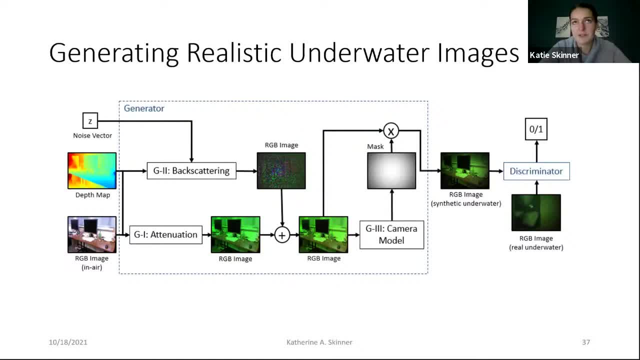 robust platforms for those types of environments. But you can also think about you know multi-robot teams where you might have. you know multi-robot teams where you might have. you know multi-robot teams where you might have a UAV or a drone platform that's helping to survey, survey an environment like that. 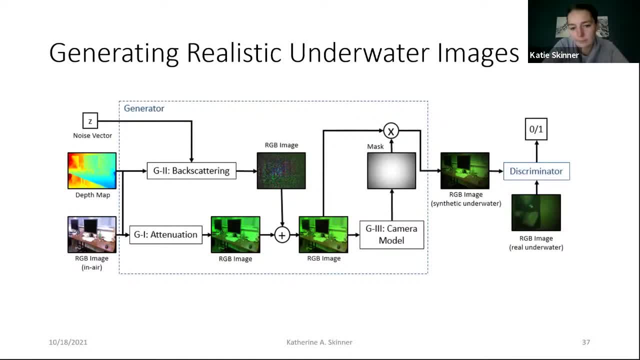 that might be more challenging for an AUV, And then the then there's interesting perception problems that come in there, where where you're trying to merge mapping information or or perception information from these different platforms that that move in different ways, and 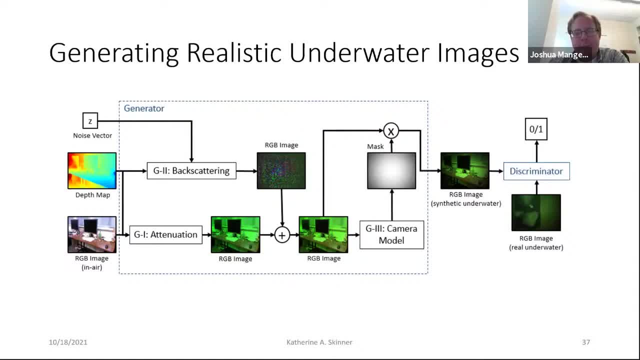 potentially perceive the environment in different ways. So I think, yeah, that seems like a lot of exciting research and technical challenges, or even system building challenges, both for such platforms. Yeah, definitely, Yep, Okay, I guess there's one more question on the slide that you are on currently. So What were your? 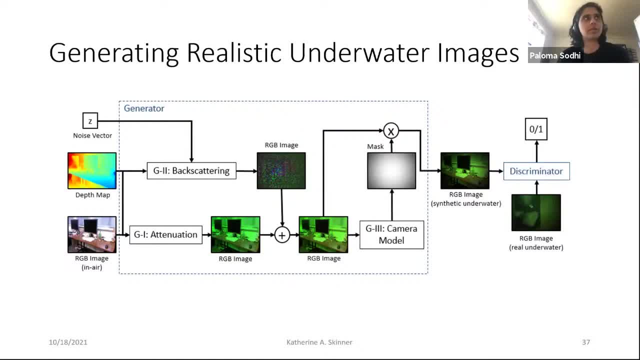 observations with the structure generator. Like, was the structure generator more stable than what a general GAN would be? Yeah, So that was, yeah, a nice kind of outcome of the structure generator was easier to train than typical GANs- can be pretty unstable, So that was definitely one nice benefit. 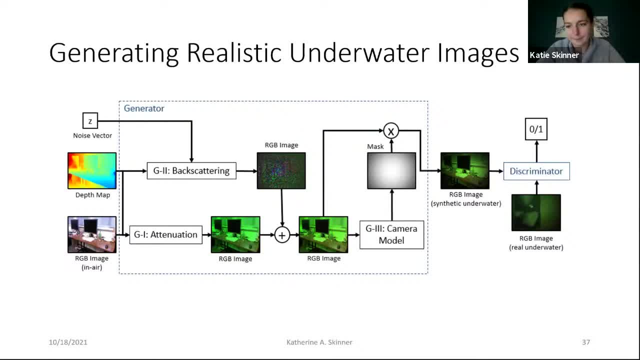 of structuring the generator this way, Maybe like, and that insight transfers across. going back to the one of the questions we had earlier, two different, Yeah, I think. anywhere you can add, you can add structure, especially, you know, structure that's based on our knowledge of. 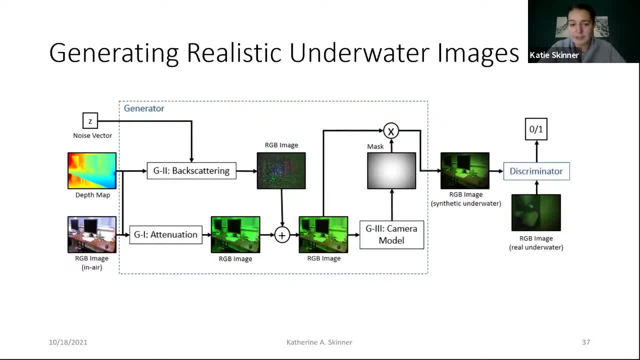 the problem we're trying to solve. anywhere you can add structure or constraints from our own knowledge and experience can be a really useful, a really useful way to think about designing deep learning frameworks. So I have a. I have a quick question too. so usually when you incorporate, 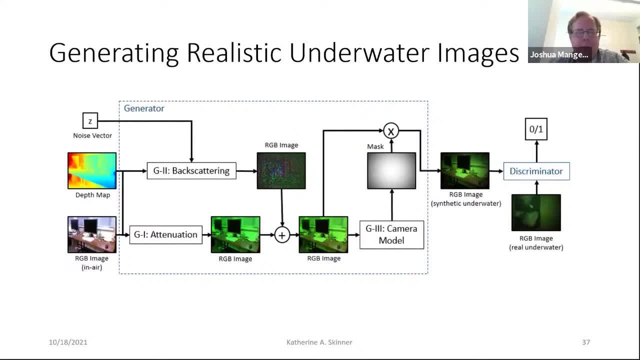 structure like that. it enables you to be able to generalize more easily, right? because because you, instead of learning for a specific situation, the, the structure and the mathematics goal theory behind it tends to localize you, to be able to generally to not change much of the network, and so you end up with something that generalizes more easily. Do you have any thoughts? 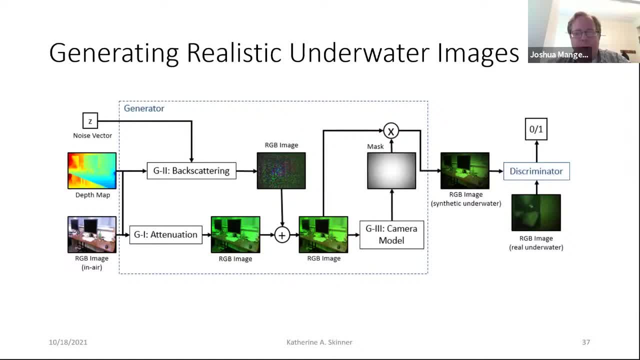 about how you would, how you could make something like this more generalizable so you don't have to train necessarily parameters every time. Yeah, I think one challenge here is just access to data from different environments, so we never tested, just training the network on a wide range. 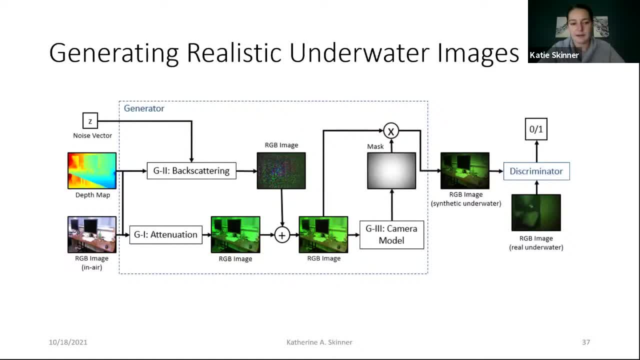 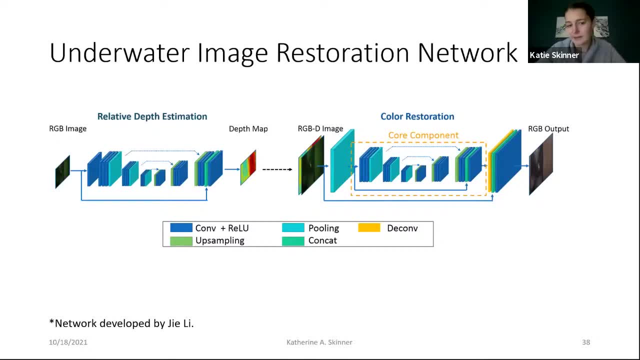 of RGB images, but I think that could be. that could definitely be possible, and especially for the underwater image restoration network, I think if you had a really large synthetic data set that you had generated from different underwater environments, I would hope it could. it could learn to output more of a generalizable image restoration process, but that was something we 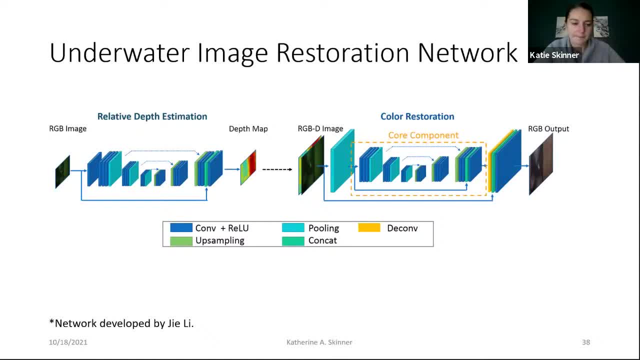 didn't test specifically for this network, because we were. we were focused on learning the parameters for specific environments, to study a local, local area, And also probably due to the lack of data, right, but it's. it's difficult for this project when we started, certainly, but there's been a lot. 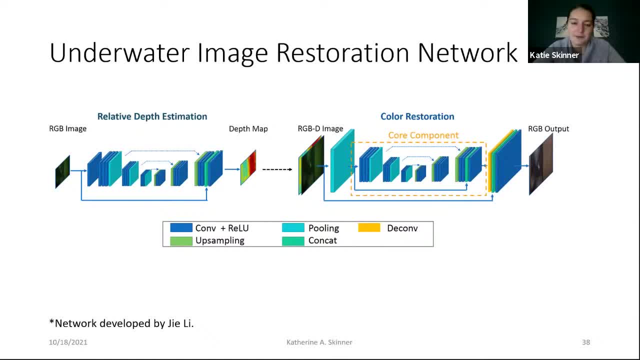 of really exciting work now in deep learning for underwater image restoration and a lot, of, a lot of the recent works can learn generalizable image restoration across different environments. Maybe one quick follow-up to like what Josh just thing. so when I was looking at your thing I was wondering: 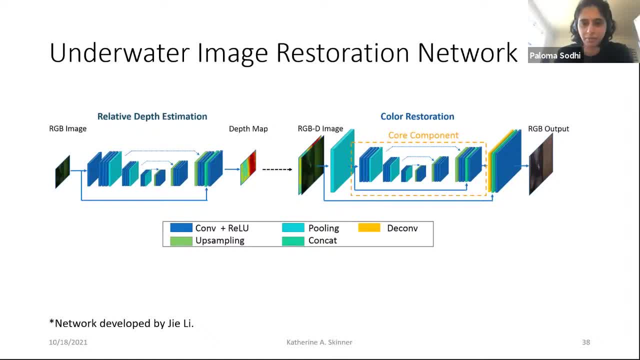 like, it's fundamentally a low data regime, which makes it an interesting problem from both learning and model-based side. but like, have you like? there are some recent variants of GANs which would use, like more unpaired image image data to sort of learn some sort of like style transfer of. 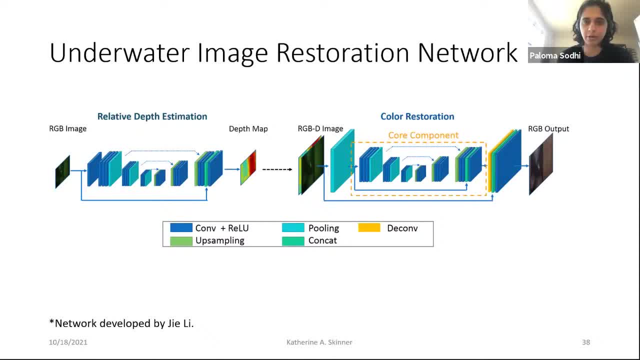 one domain to another domains. do you see that being relevant for your application? Yeah, I think some of the ideas where it's separating the style and the structure of the images could be interesting. I haven't tested it in a while but when I did test the those types of networks a 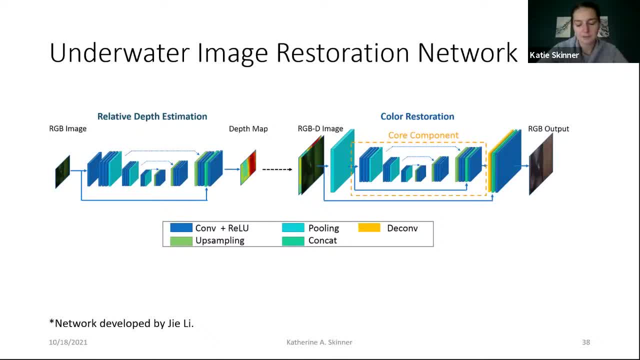 couple of years ago I still, you know, there were still challenges, just because the underwater domains and this structure of the underwater images is so different from the in-air images. so I'd be curious to see if kind of the more recent advances could overcome, overcome that. 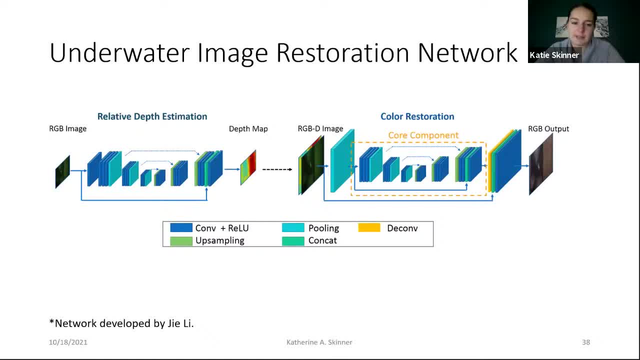 Gap, especially with separating the style and structure components, you would hopefully see that the style would align more with the underwater effects and transferring those Right, hopefully it generalizes also, then better. That's always a question. Okay, awesome. yeah, this has been a great talk and a. 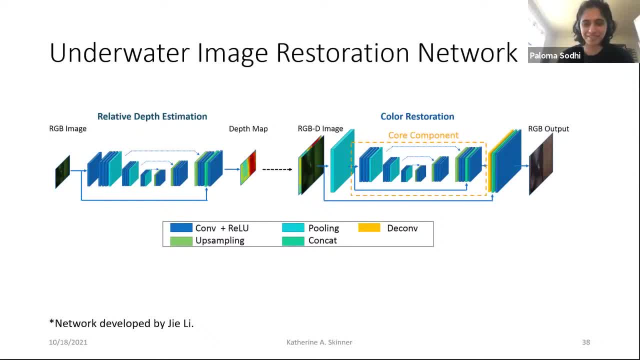 very great discussion section. thanks, Josh, for pitching in as well your thoughts on this, And thank you so much, Katie, for your time and coming out here. I think we can probably end at this. Thank you so much for your time. Thank you. thank you and Josh. 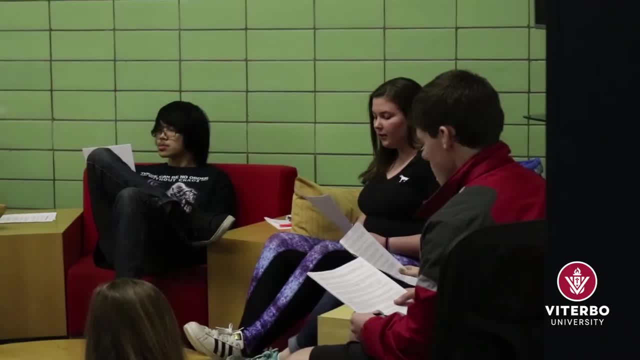 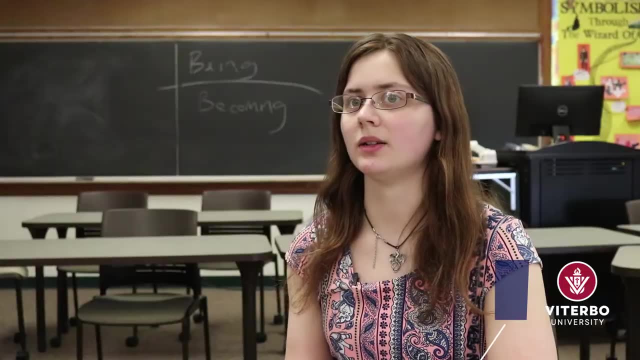 Some of the groups are talking about gun control. We had one on cloning and what that looks like, on like people versus animals. My group's doing the graphic novel Unflattening and so we're looking at it kind of through the lenses and asking the questions about it. It's a really interesting. 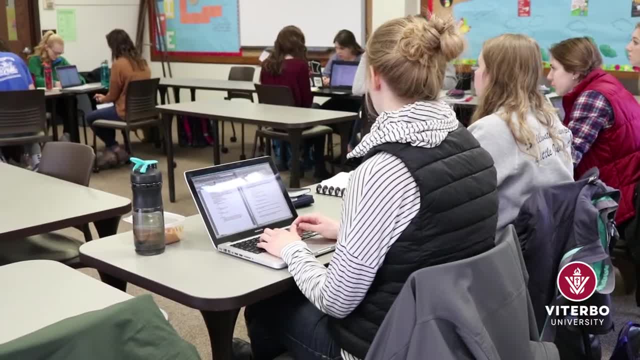 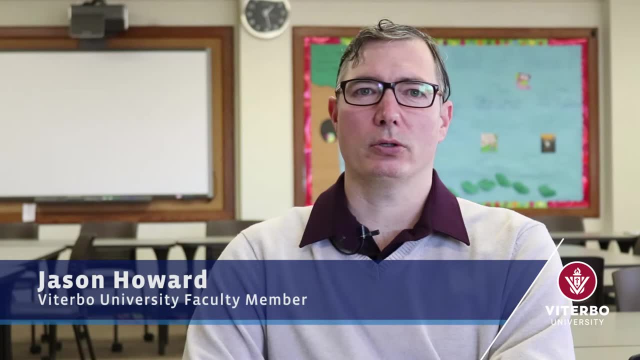 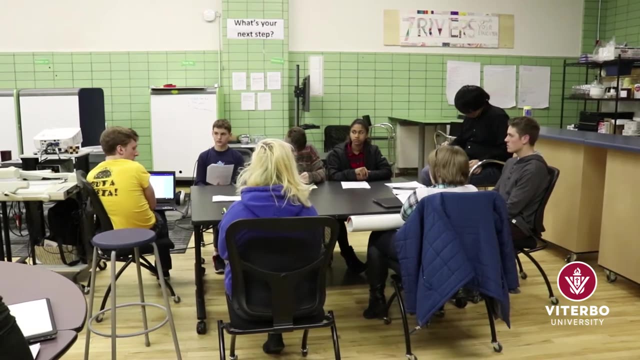 social critique, So VUSM course, Classical Conceptions of the Common Good. It's basically an ancient philosophy class that I restructured, revamped to include a service component, and the service is philosophy for children and our service is to go into the schools, and we do this from. 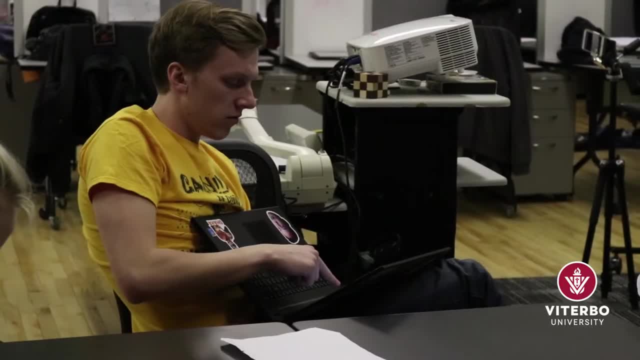 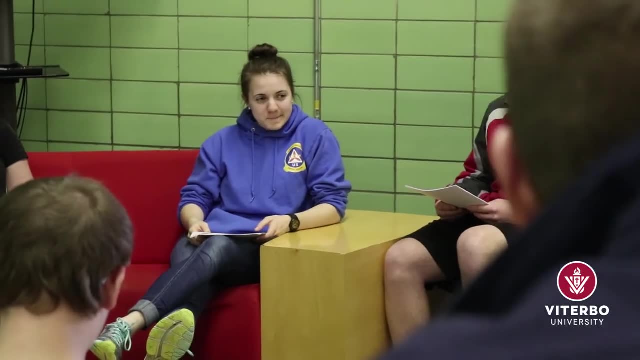 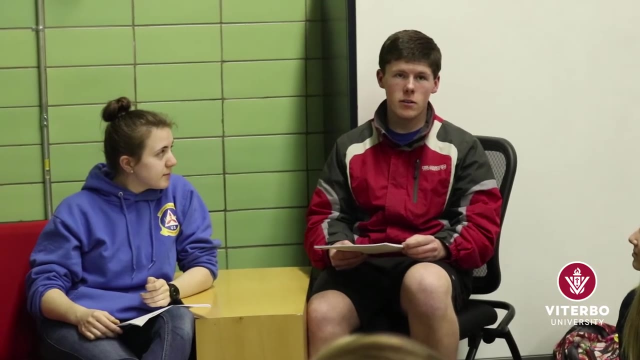 grade 4 up to grade 12 in the local charter schools and I have my students introduce philosophical problems. There's a lot of techniques, things the students should do, things the students shouldn't do. One of the great things about the program is it's really run by the kids in a way that 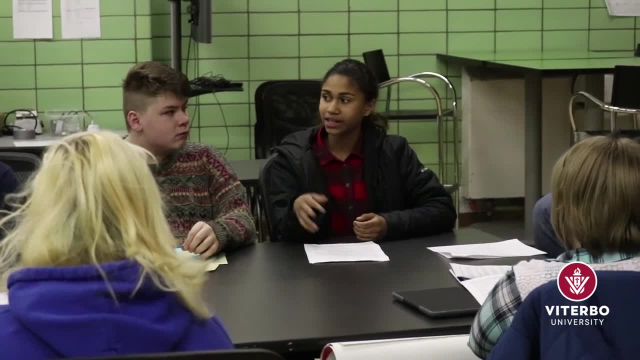 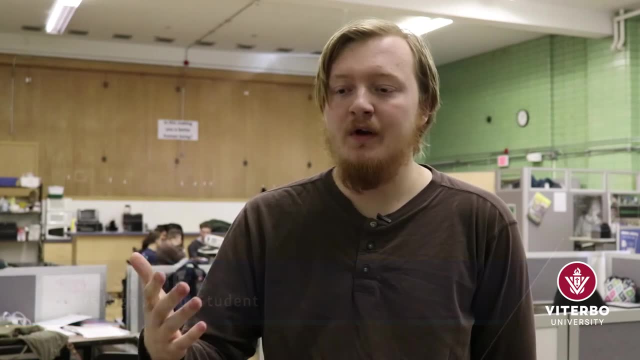 they create the questions for the conversations and it grows from there. Two things I'm taking away: One is improving my ability to talk and to talk to other people about what I believe, and the second one is not only constructing my own beliefs, but also being willing to change those beliefs based on. 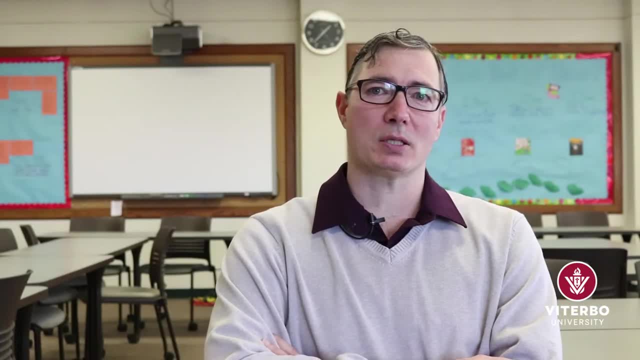 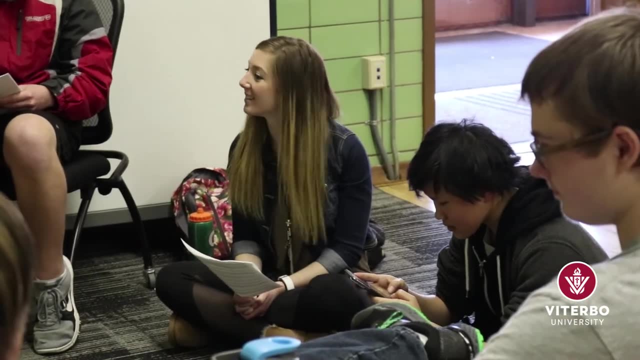 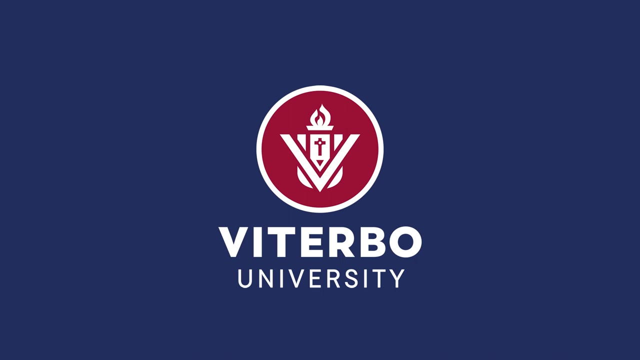 certain things that I hear Most of the time at the end of the class, people begin to kind of see that philosophy is really quite a powerful tool to just improve people's pro-social discussion abilities. We have a lot of issues and a lot of philosophy. So the first thing I wanted to say was: we really believe that there is political justice. I think, if we go off of what I said, people always want to sit there and see what they think about politics and they'll say: of course, you're right. 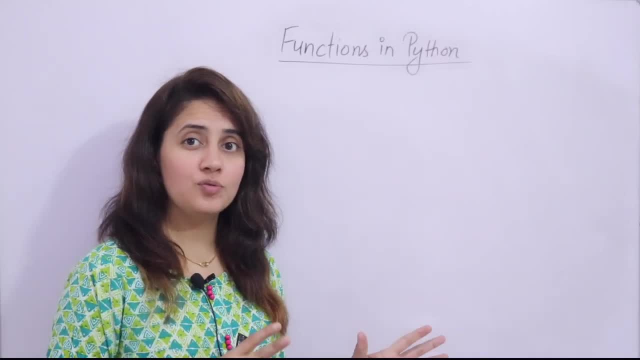 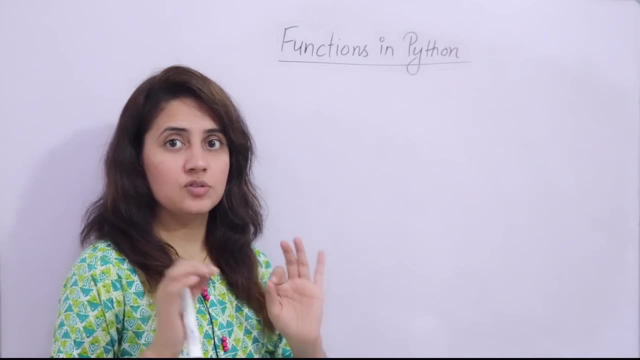 So in the series of learning Python programming language, in the previous video we have seen a project, we have created a project- hangman game right. so from this video I'm going to start a new topic, that is, functions in Python right, and this video. in this video we'll be discussing basic.